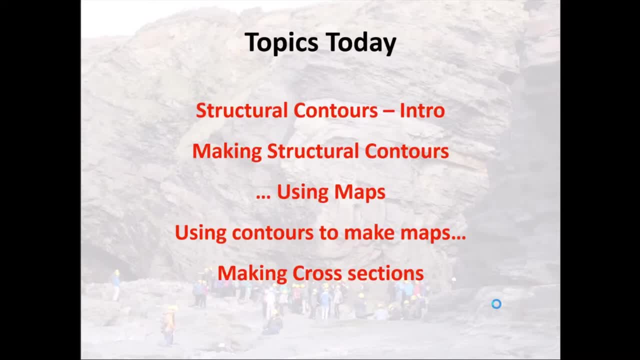 angle of dip some inclination. Today we're going to cover structural contours and show them how they can be made using maps, and then using structural contours to, in turn, make interpretations about maps. and then we'll show how we can use structural contours to make cross sections for dipping rocks. Okay, hopefully you guys remember that we've been talking. 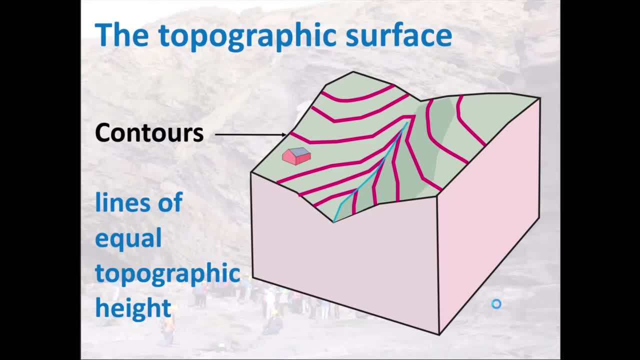 about contours in terms of topography, and contours are just lines on a map that join points of equal height. That's what a topographic contour is. So you can imagine on our block diagram all of those lines that we can see on the top surface of the block diagram. they're 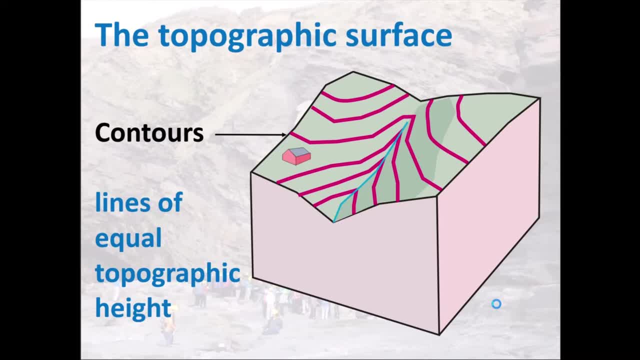 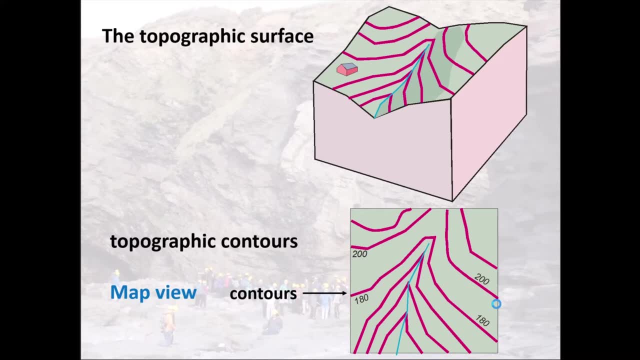 joining points of equal height above sea level. and if we were to look at that- the top of that block diagram, in in map view, Then this is the sort of map that we'd generate. This would be our map view and these red lines they'd be our contours: joining points of equal height above sea level. 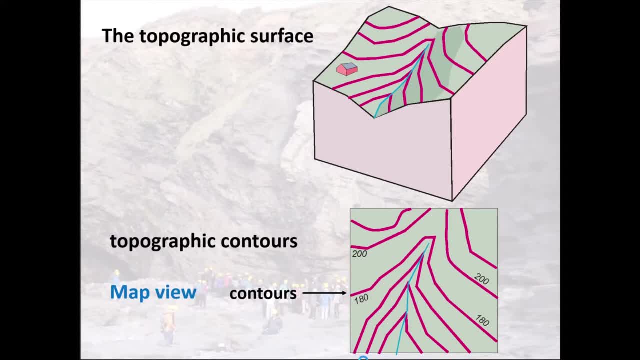 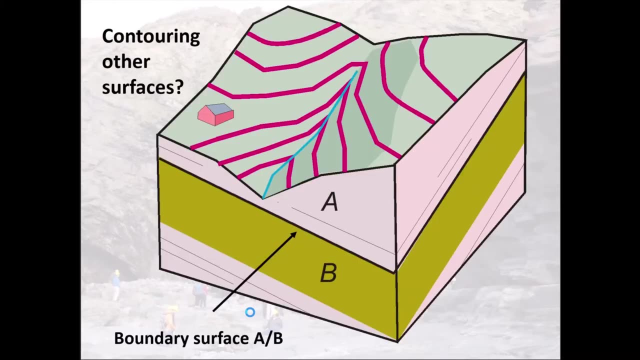 So, if you think about it, all a contour does. all the topographic contour does is show you how height is varying along the surface Right. so why then can't we draw some contours for other surfaces? Let's imagine that we have these two sedimentary beds, A and B, and between 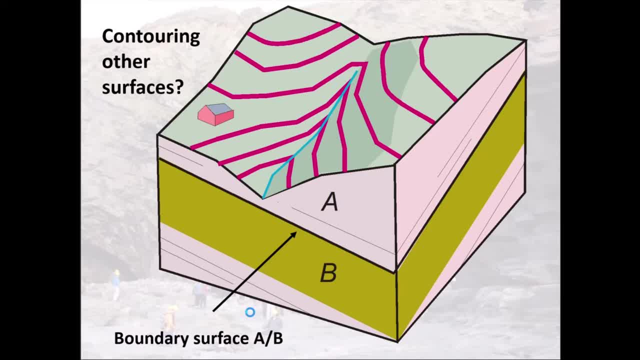 them. there's a boundary, there's a bedding plane, and let's call that surface AB, That plane that separates A from B. Let's imagine that then we could lift off that rock unit A. We could just like scoop it off the surface to expose that plane. 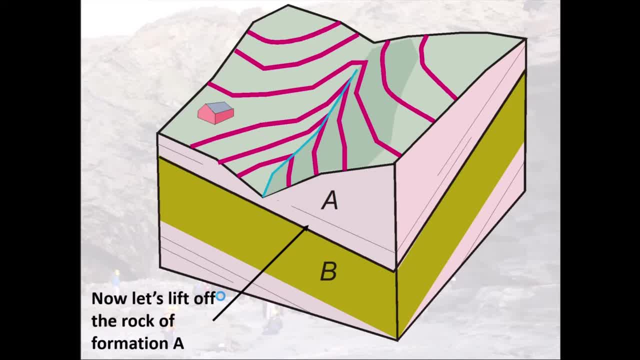 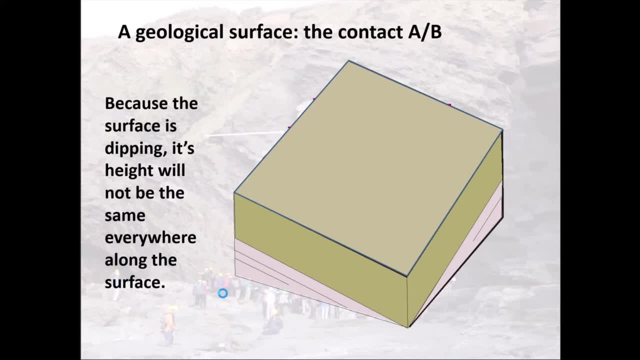 Okay, Let's take A and remove it from the surface. Let's just lift it off so we can no longer see it. Now we're looking at that surface, that contact AB, that plane that separates rock unit A from rock unit B. 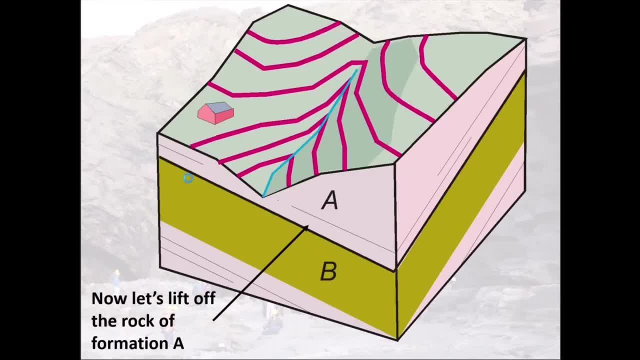 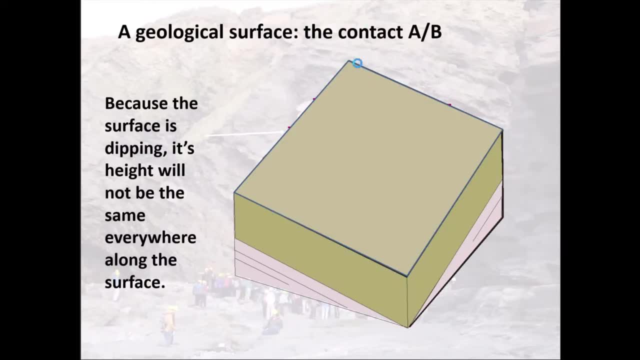 Now hopefully you guys can see that this plane, this AB plane, it has a dip to it. It's kind of it's dipping down towards us. in effect, It's high over here and it's low over here and it's sort of dipping. 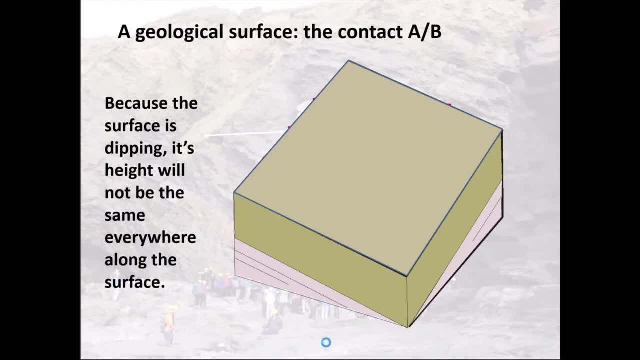 It's going down in this direction, Okay, and because it's dipping, the height along that surface will not be the same everywhere, Like if you were to be sat on it, you'd be higher up than if you were to be sat down here, Okay. so, for example, the up-dip surface will be: 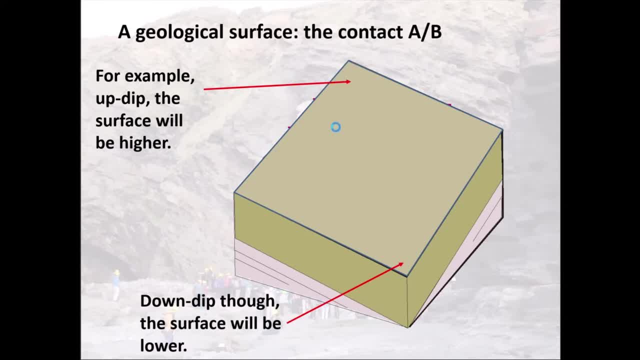 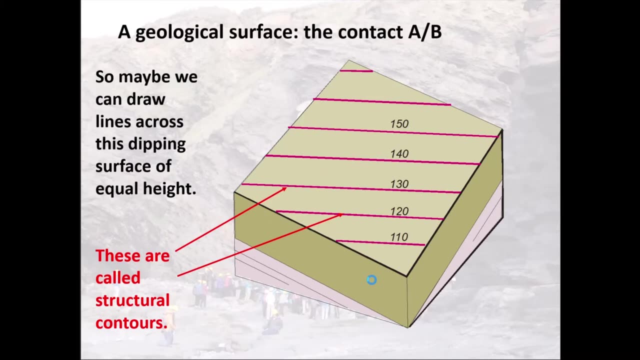 higher. It'll be higher above a sea level or whatever datum we use, and the part of the surface that's down-dipped, that's closest to us, will be lower down. So maybe what we could do then is draw lines across this dipping surface of equal height. 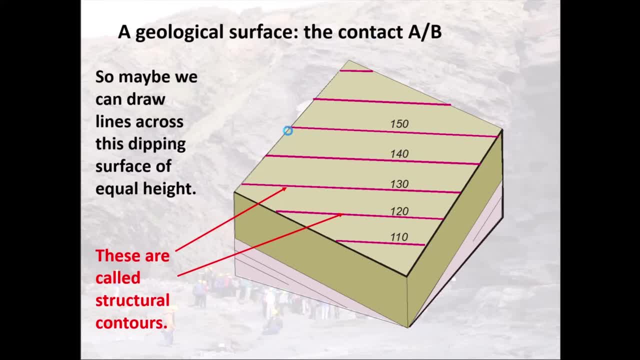 We can draw contours. So, for example, if we were on this dipping surface and we walked along it in a horizontal line along this, we'd always stay at 150 meters above sea level. That line along that surface. AB would connect all of the points along that surface where 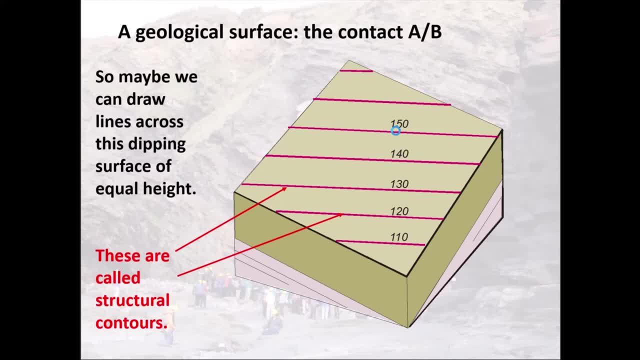 the height is 150.. Okay, It's just like a contour, Because we're drawing contours on a structure, in this case a bedding surface. we call this type of contour, we call them structural contours. Okay, so you can imagine. we could take those structural contours, we could look at them. 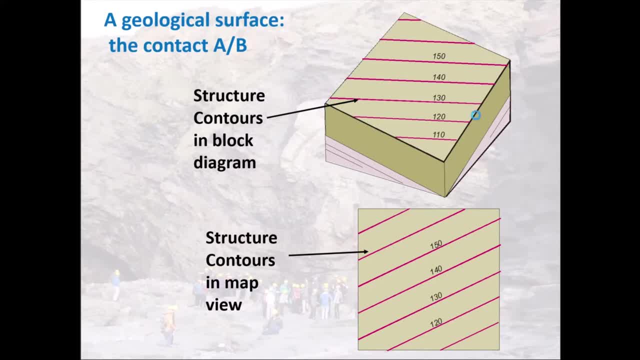 in map view- sorry, in block diagram view in three dimensions. and if we took a top-down view Of that surface, we could see our structural contours in map view, Yep, And that map would show us the height of that plane that contact AB in two-dimensional. 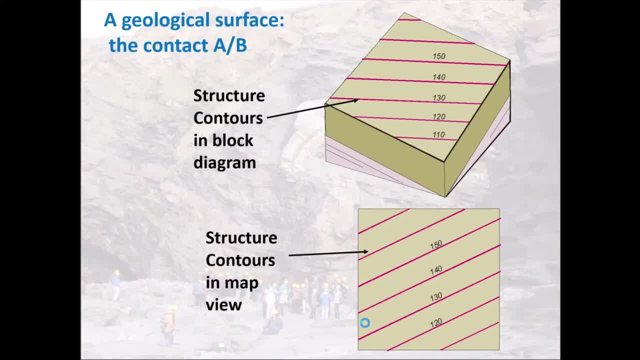 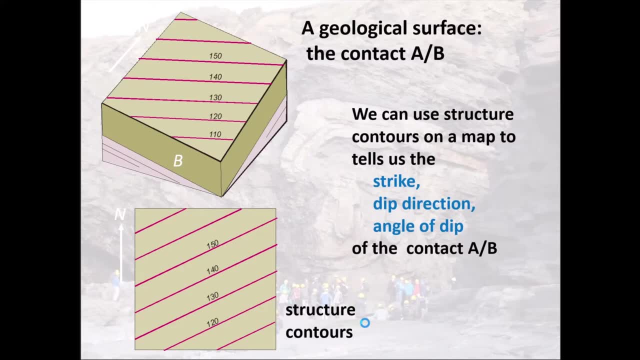 space. Now, structural contours are handy for one reason, and that's they can tell you about the orientation and dip of the plane or the feature that you've drawn on that surface. Okay, So that's that. Okay, So that's what the structural contours for. 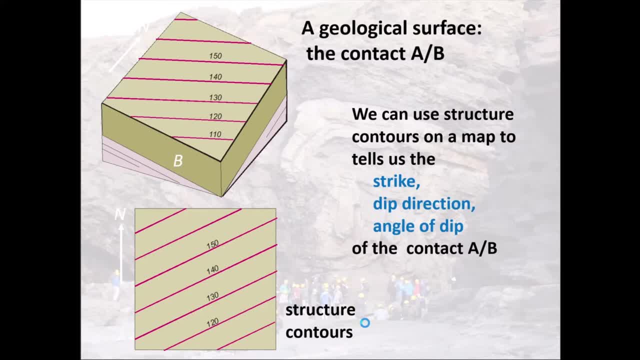 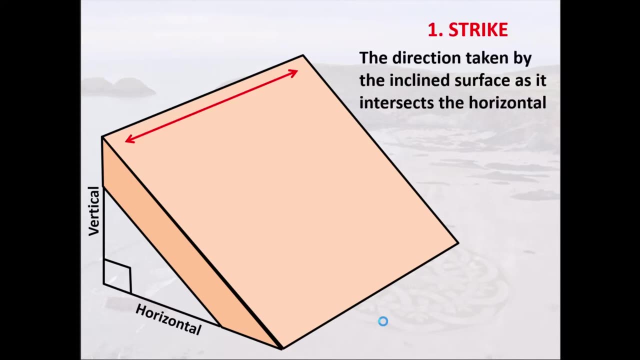 Hopefully you guys will remember that- an inclined surface, a bedding plane or a fault plane or unconformity- they will have three components. The first component is the strike and that's the orientation at which you can draw a horizontal line along that plane. 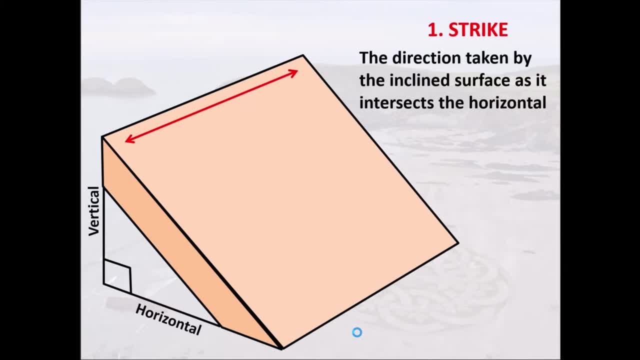 Okay, If you have an inclined surface, there's infinite numbers of lines that you could draw over that surface, but there's only ever going to be one orientation where you can make a perfectly horizontal line, a line where the height of that line doesn't change. 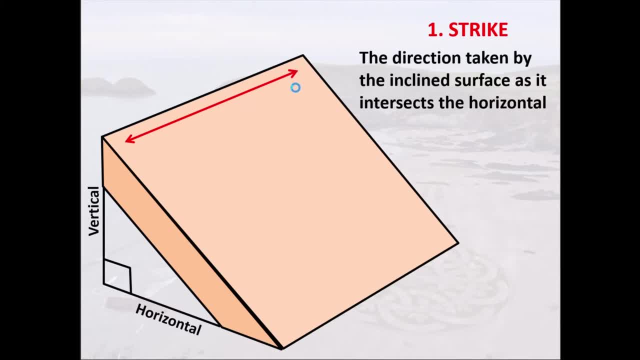 The second feature or geometric feature that a planar surface has is the dip, and that's simply the angle between the horizontal and the dipping surface. Okay, that maximum angle from the horizontal down to the dipping surface, And then the dip direction. The dip direction will be the compass orientation, the bearing in the direction of that dip. 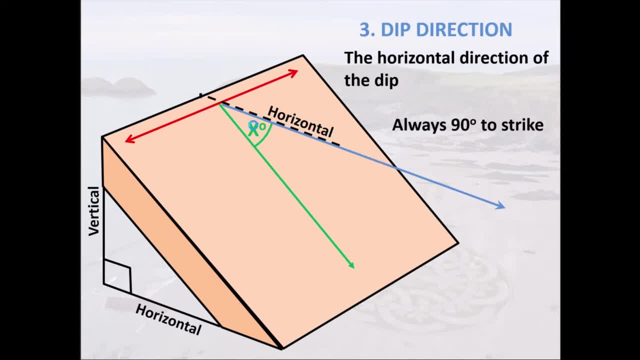 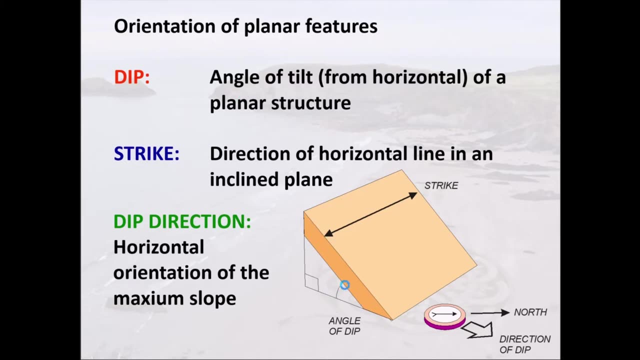 Okay, and an easy way to check whether or not you've measured the dip direction correctly is that the dip direction is always, always, always, always perpendicular to strike. Okay, so those are our three components. Dip is the angle of tilt and this angle of dip is the same as this angle of dip here. 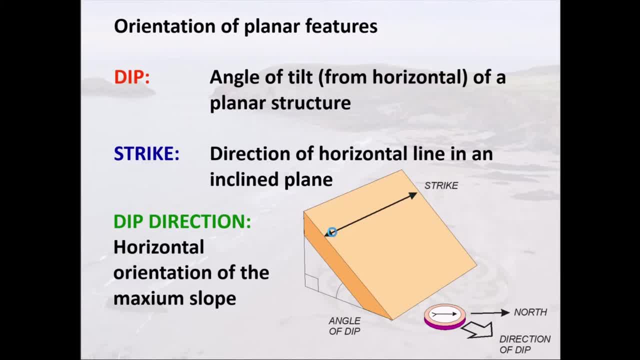 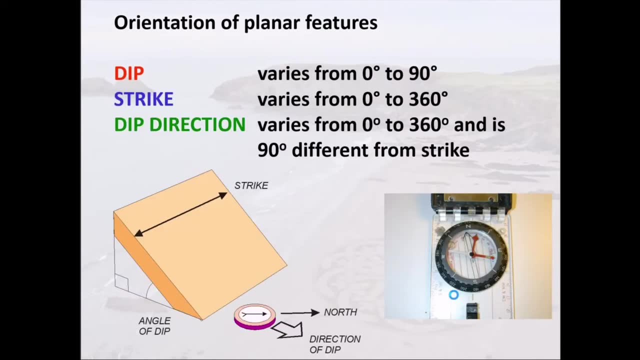 The strike is a horizontal line along that inclined surface and the direction of dip is perpendicular to strike and it measures the compass bearing in the direction of dip. Dip can only vary from 0 to 90. It can either be horizontal, vertical or somewhere in between. 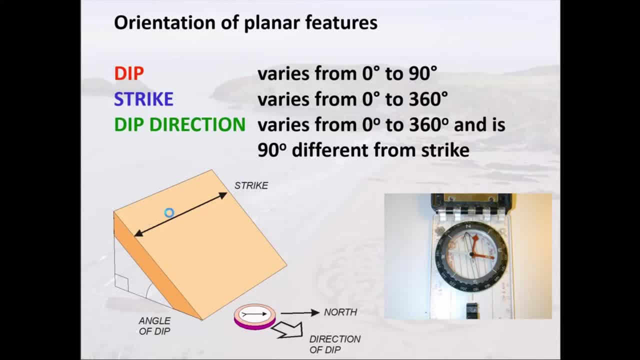 And the strike, because it's a compass orientation, like it's a direction on a map. it varies from 0 to 300.. And similarly, because dip direction is a bearing, it's a direction on a map. that, too, varies from 0 to 360, and it is always perpendicular from strike. 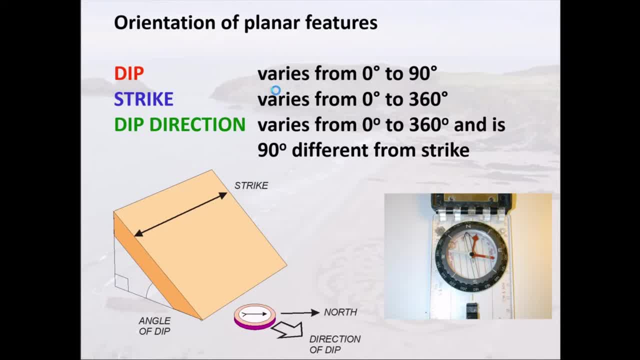 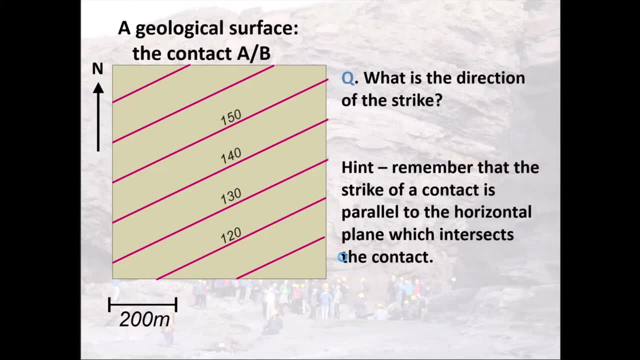 Okay, that's a refresher of the structural features of inclined planes, And then let's go back to our geological contact AB. This is our map view showing the structural contours for that geological contact, And now we're going to figure out how we can use these structural contour maps, or the structural contours in map view, to figure out those three components of inclined planes that we just refreshed ourselves about. 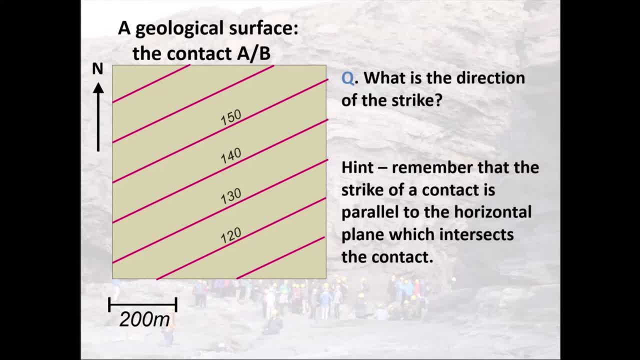 So the first one: how can we use these structural contour maps to figure out the direction of strike? Well, a key thing to remember is that the strike of a contact is the horizontal line along that plane. Okay, And if you think about it, each one of these structural contours is a horizontal line. 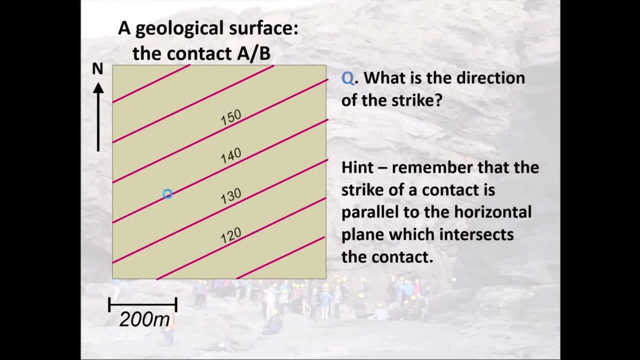 It's linking points of constant height above sea level or above whatever datum. So everywhere along this line, for example, every point along that line, the height of the plane is 140 meters above sea level, say Okay, so by definition, each one of these structural contours is a horizontal line. 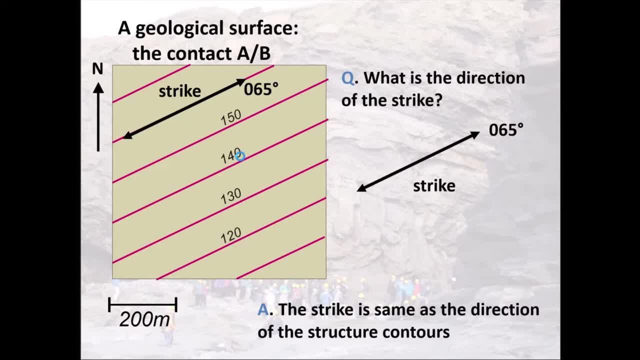 Therefore, you can simply measure the orientation of these structural contours and they will give you the orientation of strike. So strike take-home point. strike is the same orientation as the structural contours. So if your map has a north arrow on it, we can measure. 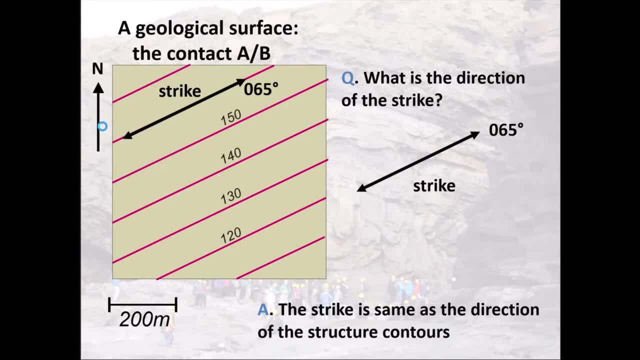 clockwise from north, that angle between the north arrow and our structural contour. When we do that in this example, we get an angle of 65 degrees which, because it's a direction, we give us a three-figure number: 065.. Because a strike for some people. it can have two directions if it's. 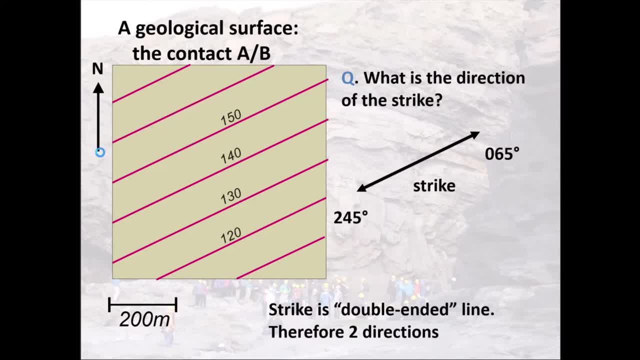 striking 065, then it's striking 180 degrees the other way, so 245.. There are such things as the right hand rule, and whether or not you agree with that as the best method to learn these things is up to you. But if you want to call strike a two-number reference, then I don't really have a massive 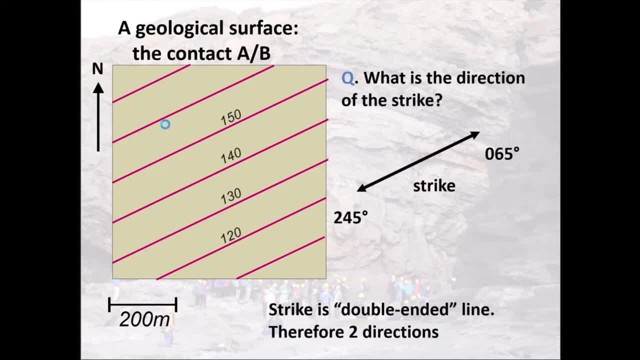 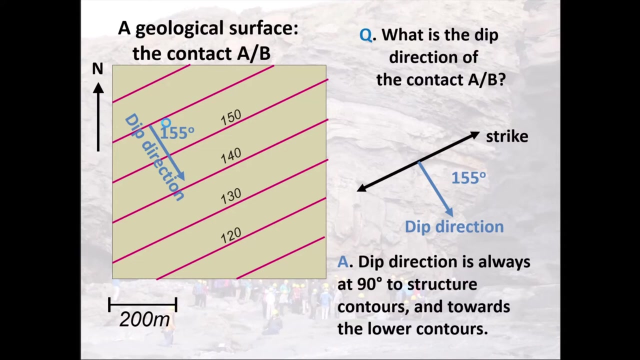 problem with it? Okay, next question then: What is the direction of dip, of the contact AB, If you think about that for a second? Well, we just realized, or remembered, that dip direction is always the direction of the contact. It's perpendicular to strike. So if we've got our strike line as being parallel to our ground, 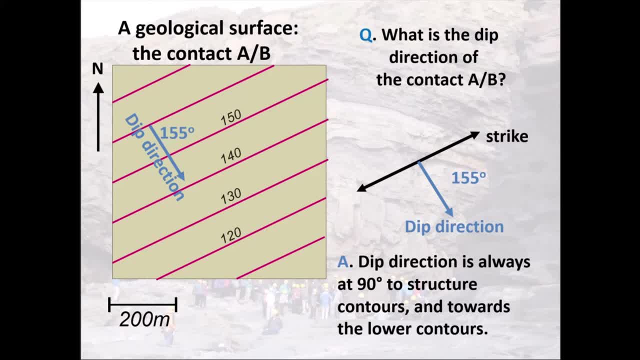 contours, then the dip direction is going to be 90 degrees to it. right, It's going to be in this direction that I'm potentially in this orientation that I'm moving my mouse, So to figure out whether or not that plane is dipping in this direction or in that direction. 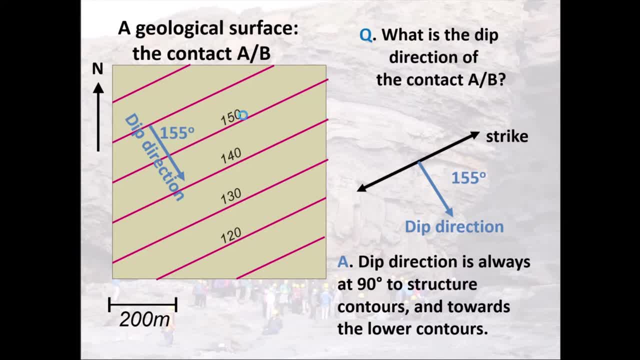 we have to look at the actual numbers on our structural contours. We can see that we're on the 150 here, 140 here, 130 and 120 down here. So we're going downhill, We're going down dip in this direction, aren't we? 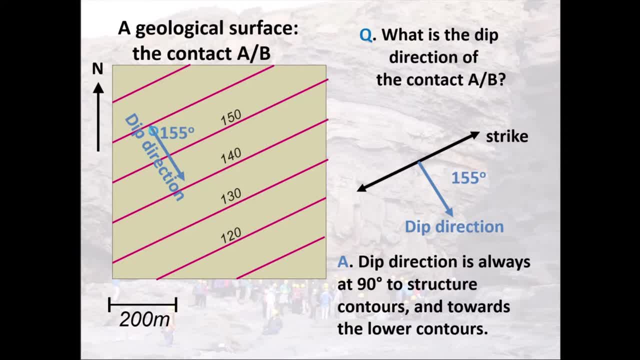 So the only dip direction that works for this structural contour map is in this direction. So to summarize that dip direction is always perpendicular to the structural contours because the structural contours are parallel to strike And the Direction of dip is always going from the higher values on the structural contours to the lower. 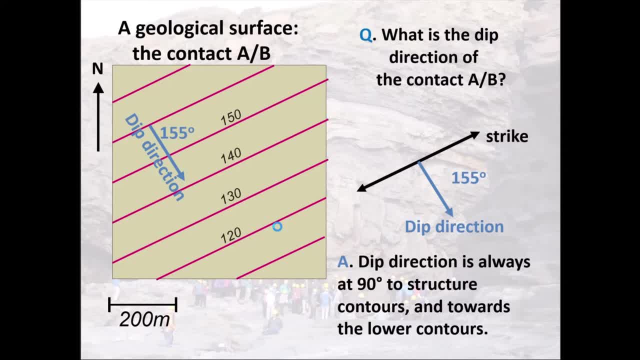 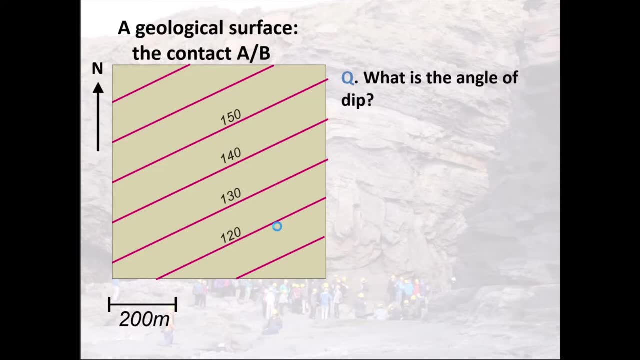 values of the structural contours. So in this case our dip direction would be 155 or southeast. And then the last component of our plane that we can measure from structural contours is the angle of dip. How steep is this plane? Now, we can't just directly measure this, We can't slap our compass on a structural contour map. 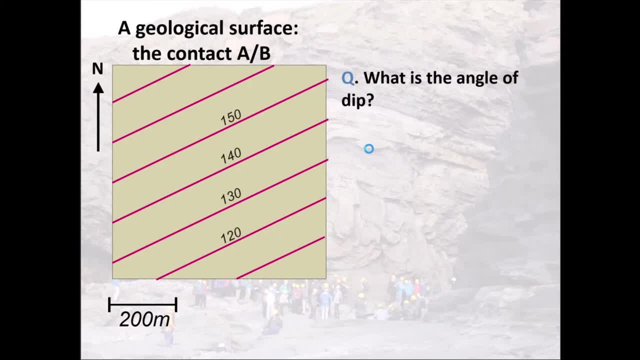 We have to do a little bit of maths And what we need to do is find two points on that plane, on the structural contours. So, for instance, I've taken a point here for 150 and then I've gone down, dip, along the dip direction, to another point on the structural contour. This one's at 130.. 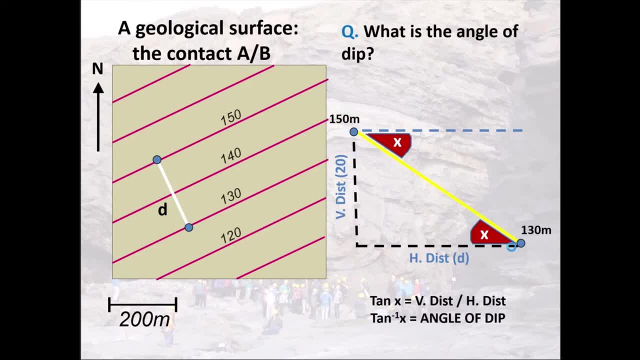 What we can then do is draw a little triangle where this yellow line is the surface AB. so we're kind of looking at it in cross section. Here we are at 150 there and here we are at 130 there. That gives us a vertical distance change of 20 meters and a horizontal distance change of whatever our map scale is at. 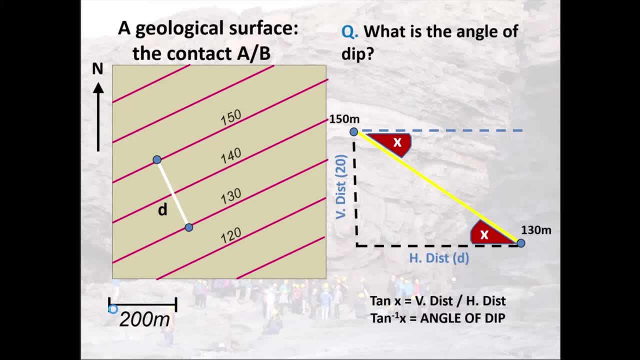 That gives us a vertical distance change of 20 meters and we can then właści menu the horizontal distance change of whatever our map scale is and we canне scale is okay. so once we have our vertical distance change and once we've calculated our horizontal distance change using our map scale, we can then 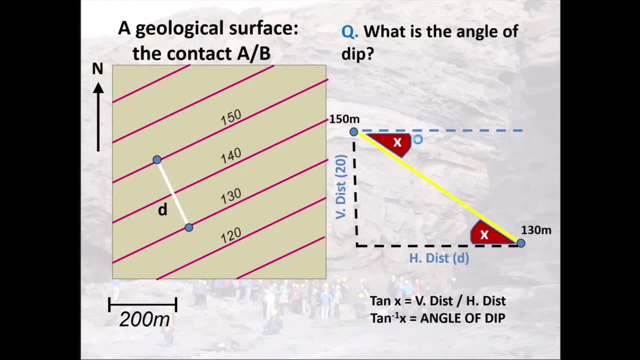 work out that the tangent of this angle X, which is the dip, is equal to the vertical distance divided by the horizontal distance. once we have that ratio, we can take the inverse tangent of it and that will give us the angle of dip in degrees. okay, so maybe just practice this in the lab. a couple of 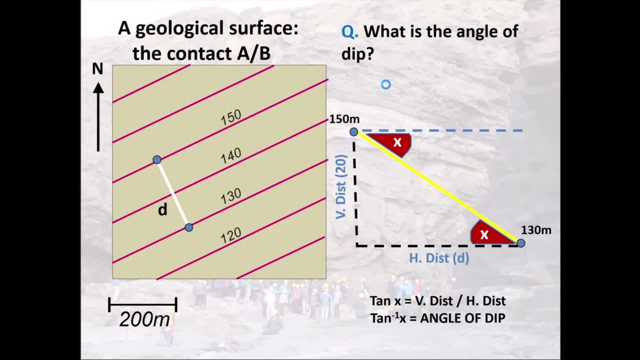 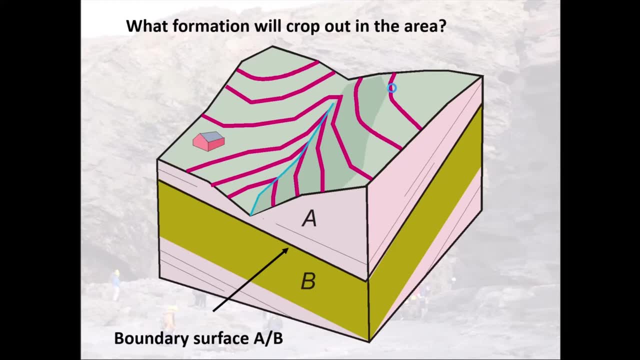 times, just so you know what the mathematical orientation is. okay, let me now ask you guys a question. if we were to look at this block diagram, and let's imagine that this block diagram is our entire universe at the moment and we're currently self-isolated at home, 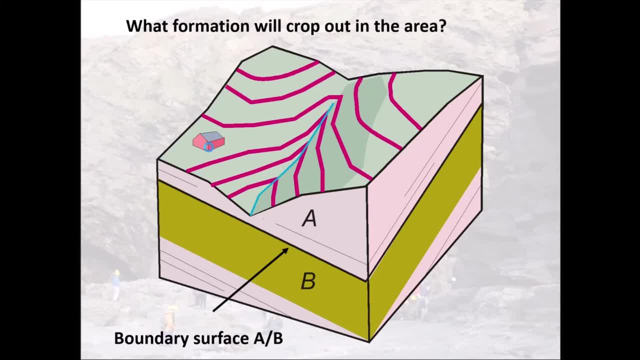 in Europe today. but my final question would be: how do we manage to work out? acordo, I think if we work out what to work out, when we put our focus to lock here, if this is our entire universe, which formation will crop out in the area A or B, or A and B? well, if you look at the map, A is the only formation. 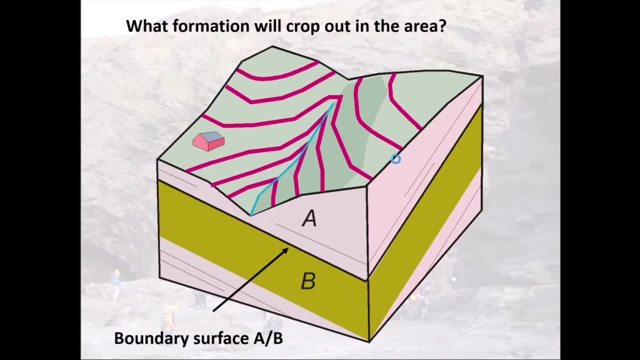 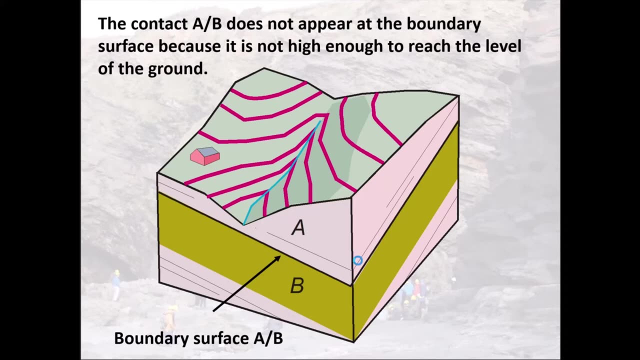 that's ever going to crop out in this area. right lonely ever be. formation a: the reason that B never crops out in this area is that the contact between A and B, it's always lower down than the ground. its height is always less than the ground itself, or in other words, the structural contours of that plane. a, B. 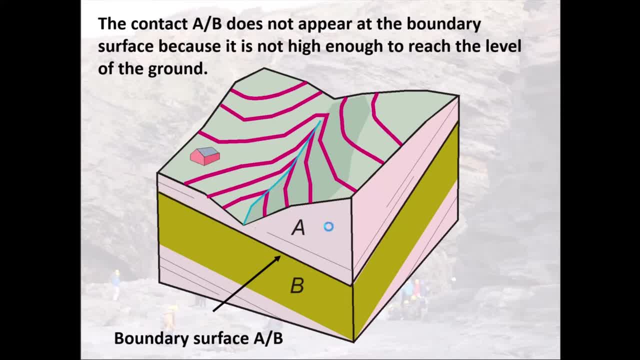 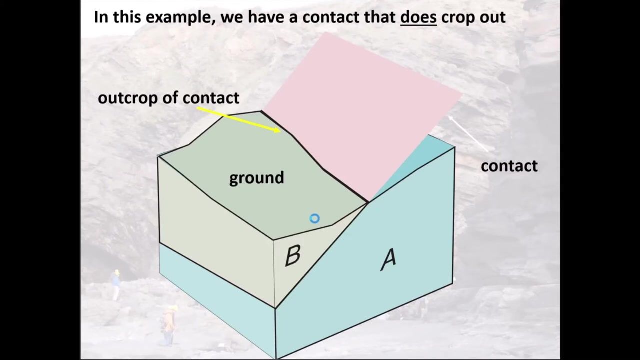 they're always, always less than the ground contours. okay, so let's keep that in mind. for A and B to crop out on the surface- the structural contours for that plane, a, B- they must exceed the ground contours in order for it to get to the surface, okay. 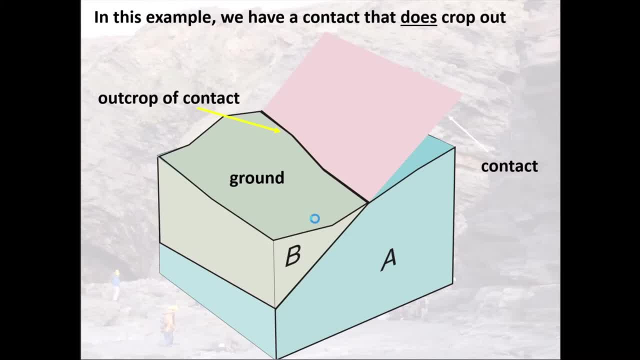 in this example we've changed it slightly. here we have two different rock types. we've got rock unit a and rock unit B, and then we've got this plane between them and in this instance you can see that the contact actually reaches the surface. okay, it breaches the surface, and 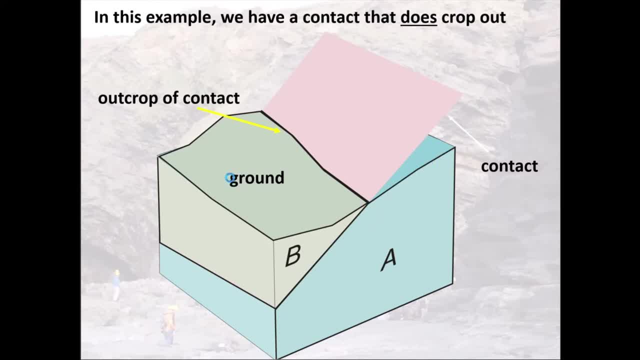 consequently, we have exposures of rock unit a and exposures of rock unit B. okay, if we think about mathematically, what we can say is that in this region, this part of our map, the contact between a and b is always lower than the ground, like if we 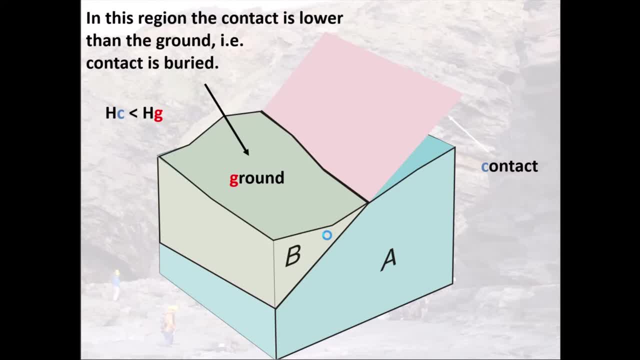 here, then we'd have to drill down to find the contact A and B. if we were stood over here, we'd have to drill down to get it. if we were stood over here, we'd have to drill down to get it in this region where B is exposed, the 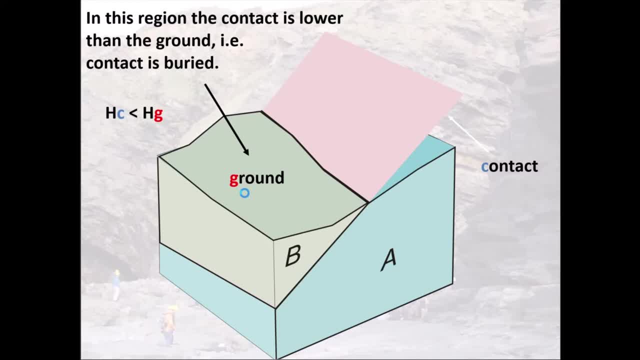 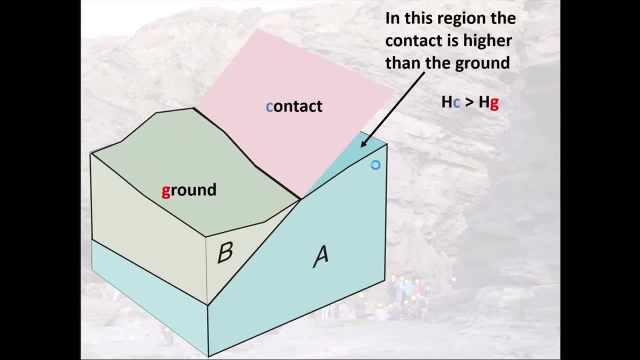 contact is always, always lower than the ground. in other words, the height of the contact is less than the height of the ground. in this region, though, the height of the contact, because it's dipping in this direction, it's actually hit. it's it's hit the ground and then it's continued up into the air. so, wherever we 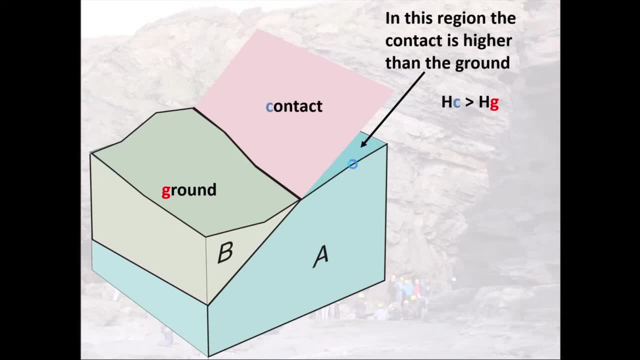 are on this side of the contact. the contact is always higher than the height of the ground. it will be up in the air- we probably see it before erosion had taken it away- but currently that contact is projecting above the ground somewhere. so, mathematically, the height of the contact is always greater than the 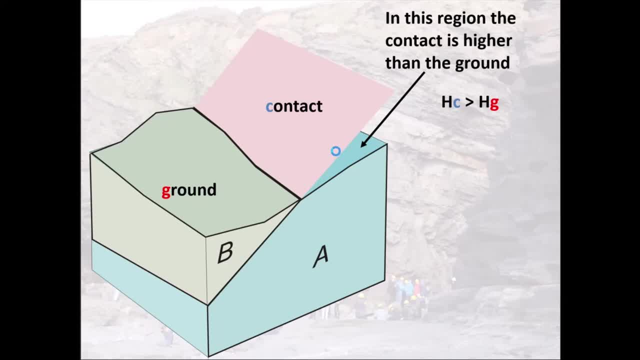 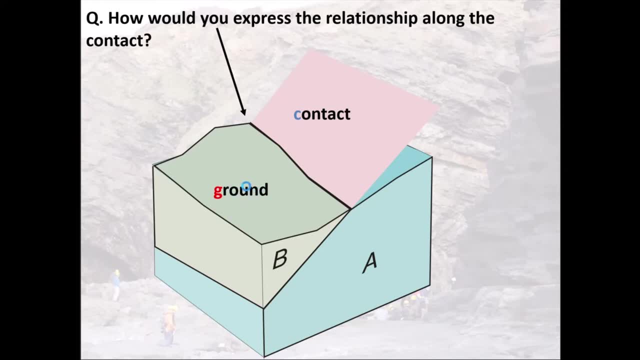 height of the ground. so if the height of the ground is higher than the height of the contact here and the height of the ground is lower than the height of the contact in this region, then how would you express the mathematical relationship along the contact, like that point on the earth where you can see that contact, where you 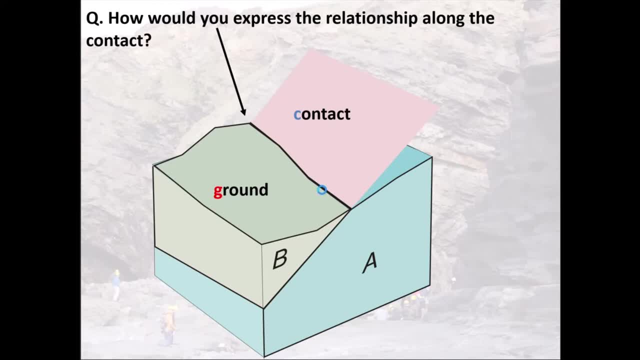 can put one foot on B and one foot on a mathematical relationship. how would you express that? well, the mathematical expression for that contact along the contact that you see on the map, is telling you that the height of the contact along that line is equal to the height of the ground. if we want to, 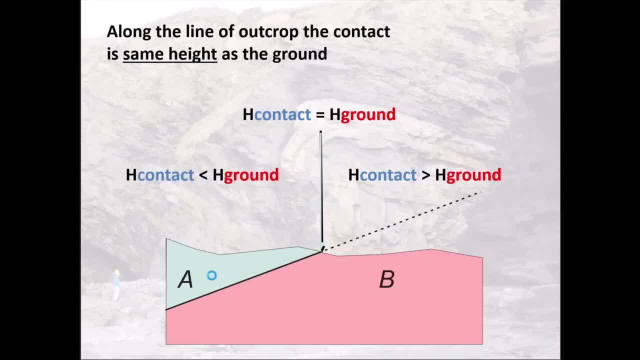 look at that in cross-section view, we can kind of summarize that over here the height of the contact is less than the height of the ground you'd have to drill down into it, and over here the height of the contact is up in the air somewhere. the height of the contact is always greater than the height of the 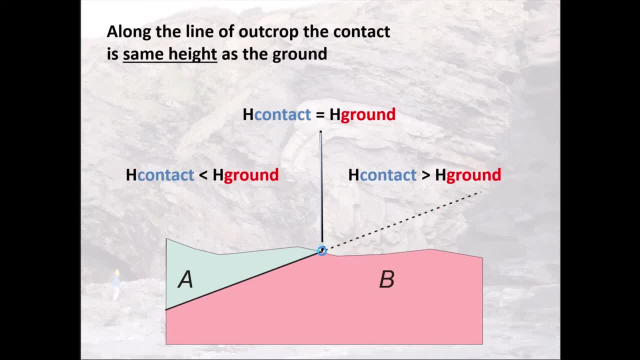 ground but along that outcrop of the contact. that's where the height of the contact equals the height of the ground. okay, if you want to replay those slides a little bit, I completely understand, but I just just want you to take away that wherever you see a contact on the 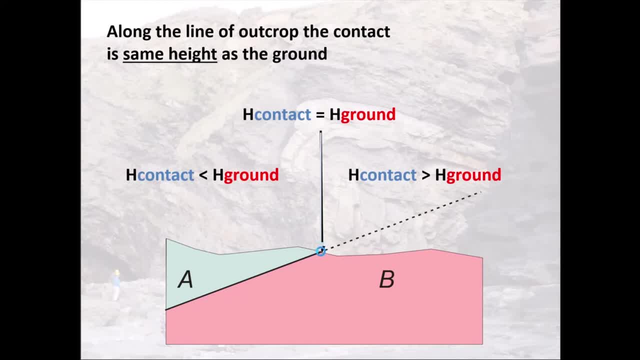 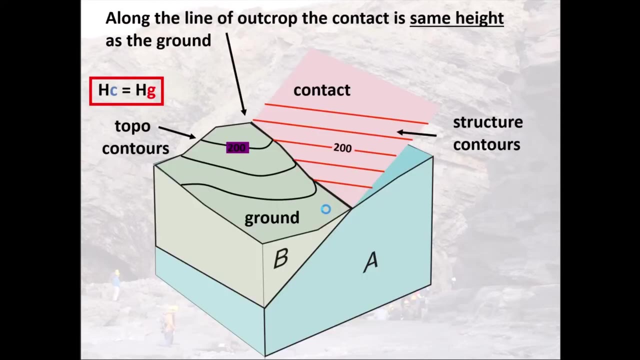 surface. the height of that contact is equal to the height of the ground. for some people it'll be blindingly obvious, but for others it may need to to replay some of those slides. okay, so if you were to draw contoured surfaces for these things, this is the 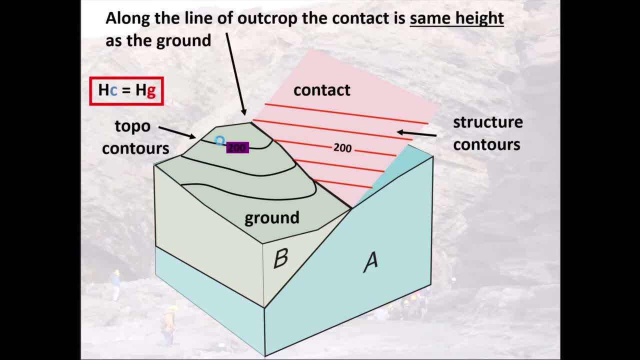 sort of thing you might end up with. these curvy, linear and contours are the topography, they're the ground surface and these red ones are our structural contours and hopefully you can see that our structural contours say our 201. here it intersects the 201 at the contact for the ground surface. 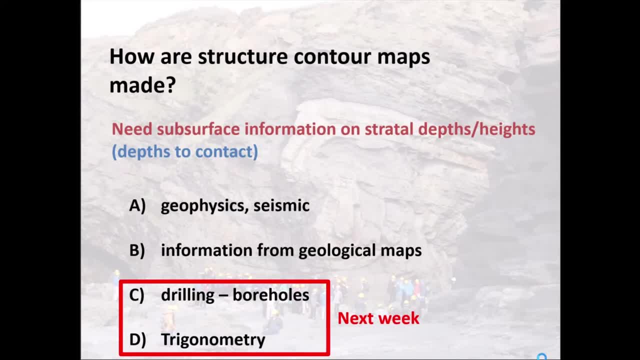 okay, so how are the structural contours of the ground surface made? in order to make these, we could use some sort of subsurface information on the depths of rocks and then figure out if it's. if it's a depth Y over there and depth X over there, we could figure out what the gradient between them is. and 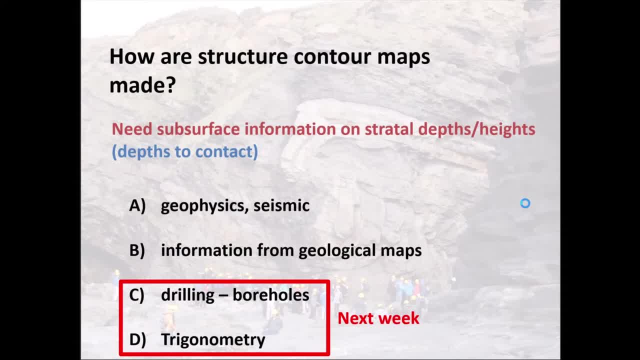 maybe we can get some of that information remotely through geophysics, maybe we could estimate it from the information that we've collected from geological mapping and maybe we could figure it out using directly sampled data through drilling, through making bore holes down into the crust to find out where rocks are at. 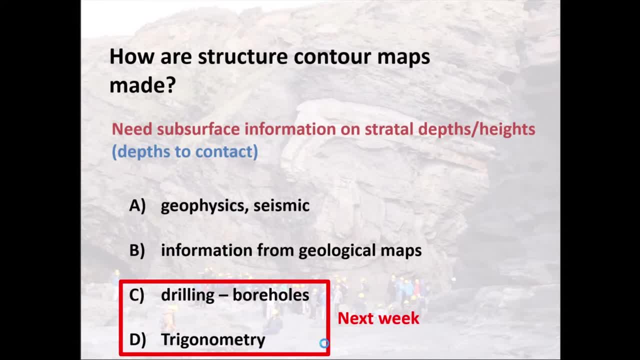 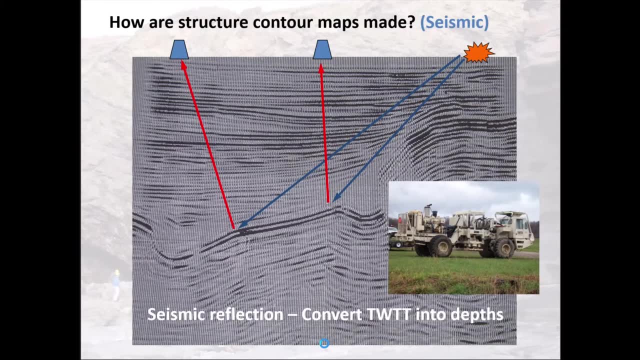 depth and maybe we could otherwise calculate it, use it trigonometry, and we'll go through these later methods next week, but maybe what we could do first of all is have a cool example of how you do it using seismic and essentially what seismic imaging requires is really an example of how you could do it using seismic and essentially what seismic imaging requires here, and this is how it's done. 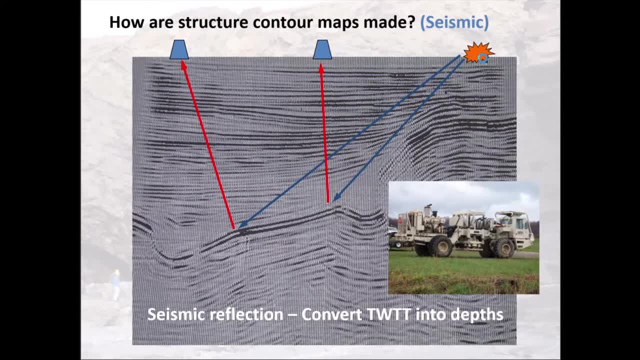 of how we could do it using seismic, and essentially what seismic imaging requires requires is a release of energy from the surface, so maybe an explosion, or maybe one of these cool vibrating trucks that sort of bounces up and down, that releases energy down into the crust as it passes through the crust when it 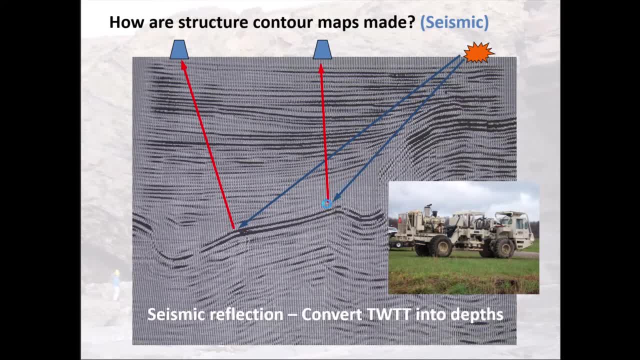 intersects a media of different density, some of that seismic energy will be reflected back and the time it takes for that seismic energy to to leave the source, hit the reflector and bounce back. when you get multiple signals from an individual reflector that does that, you can figure out the, the, the depth and 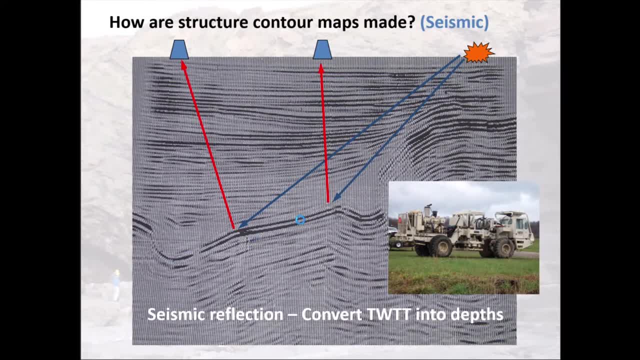 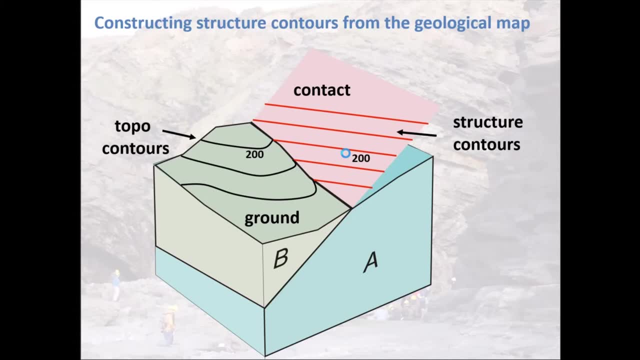 angle of the reflector of our change in bedding. maybe we could do it that way, or maybe what we could actually do is construct a set of structural contours from a geological map itself. maybe we could start with a geological map and then use where those rocks crop out on a geological map to build one. 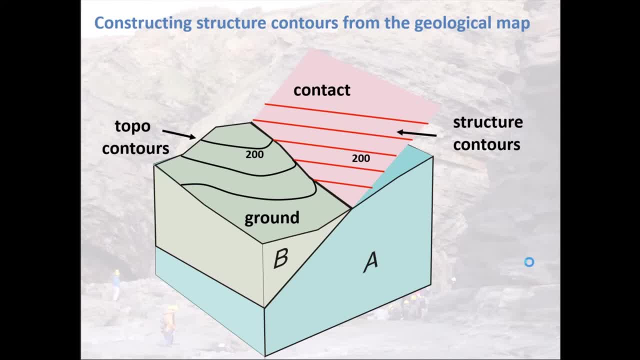 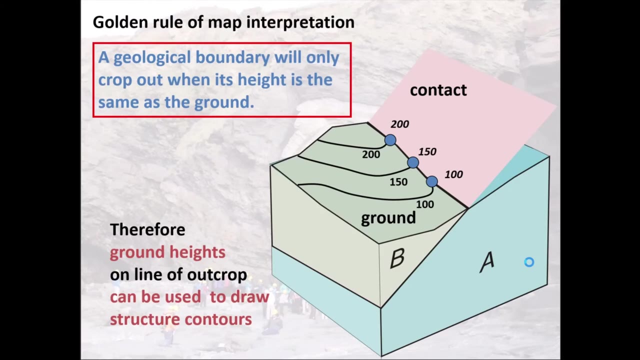 of these sets of structural contours for a dipping surface. so let's spend some time doing that. and let's start by remembering that, wherever we see the contacted surface, the height of the contact is the same as the height of the ground at that point. okay, Let's remember that. Let's write that down before we tackle the next few slides, because we're going to try and do these together as much as that's possible remotely. 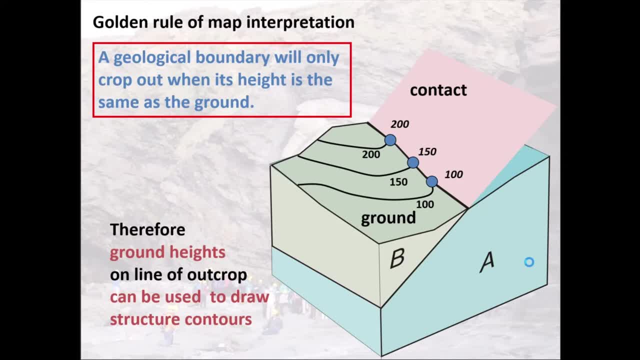 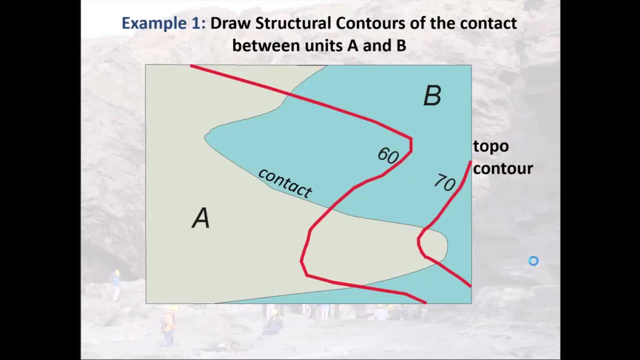 OK, so once we've got that written down, let's go and have a look at some schematic maps to see how we might start drawing structural contours. OK, so this is a map view where we've got two units- rock type A and rock type B- and this is the contact between those two units. 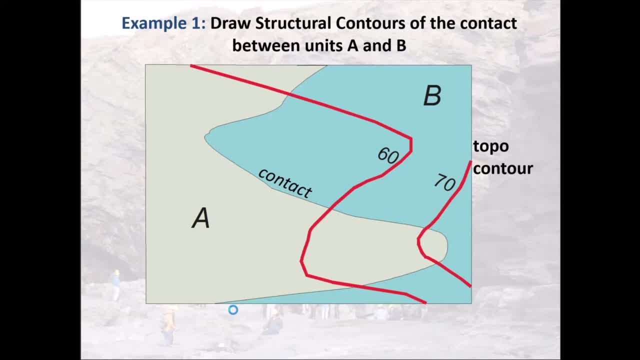 This is the plane AB. What we've also got are these red lines, which are our topographic contours, our ground heights, And we're going to use this map- no other information- to start drawing some structural contours for that contact between A and B. 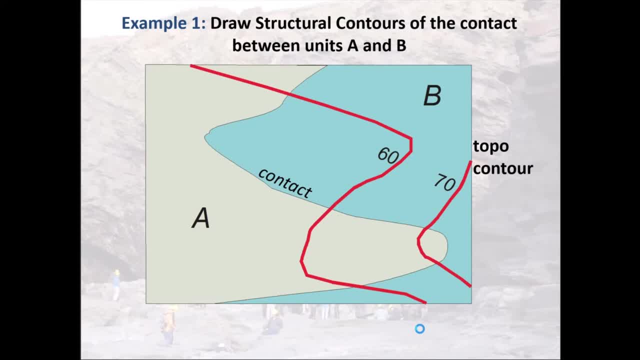 Now what we need to do is find places along that contact where we know with absolute certainty what the height is. We can give the height a numerical value. Have a think about where, if there are any points along that contact where you know for certain what the height of the contact is- 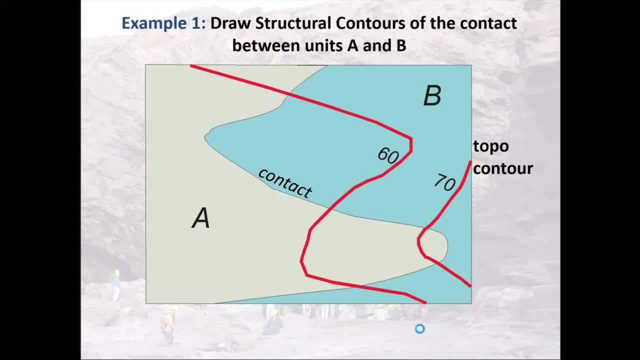 Until we know exactly where that contact is. Well, if you think about it along this topographic line, we know that everywhere along that topographic contour the height is 60, let's say 60 meters above sea level, And where our contact between A and B intersects that contour, by definition we know the height of the contact between A and B. 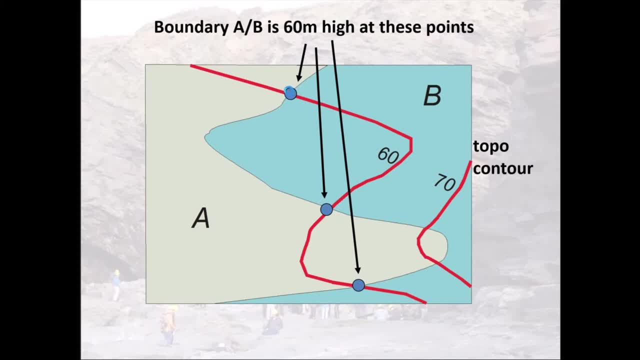 OK, contact between a and b at those points. so right here, the contact between a and b hits the 60 meter topographic contour, so at that point the height of the contact must also be 60 meters. it does the same thing there, and it does the same thing there. so then what we could do is draw a line which: 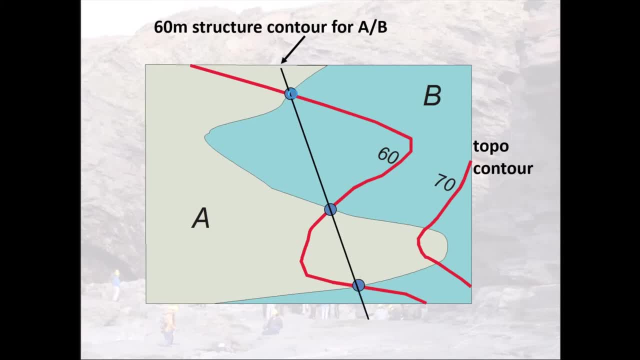 connects all of those points along that, that triplet that we've got there and that can serve as our 60 meter structural contour. so everywhere above that, sorry, everywhere along this line, that's where the contact between a and b would be 60 meters. okay, that's one line, but in order to start building a plane or to see this in three, 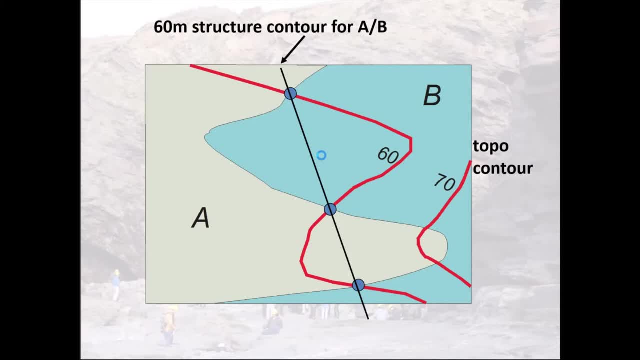 dimensions. we need another line, we need another structural contour to tell us which way we're going to be able to see this in three dimensions. so that's where the contact between a, this, this contact, is dipping. yep, so is there anywhere else on this map that we can see the? 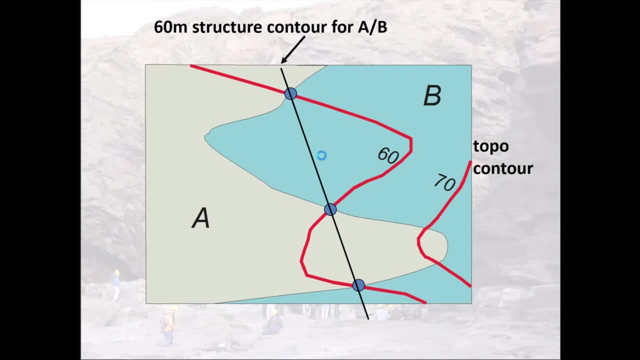 exact height of this contact a and b. well, here and here, we know that the contact between a and b intersects the 70 meter topographic contour. so at this point, and this point, we know that ground, the ground height is 60 meters. so that's where the contact between a and b hits the 60 meter topographic. 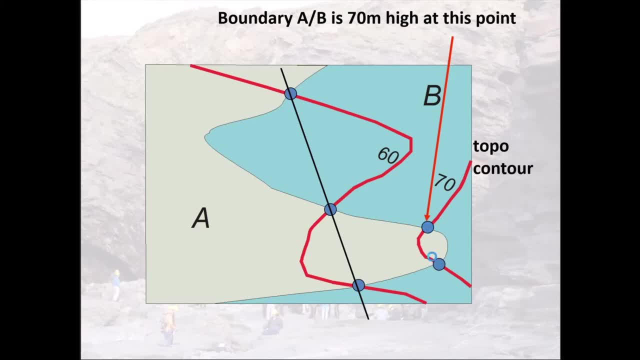 contour, so we can see that ground height is 70 and the contact height is 70, because they intersect at the same place. so then, what we can do is draw our second structural contour that shows everywhere, along which the height of the contact between a and b is 70 meters above sea level. now, 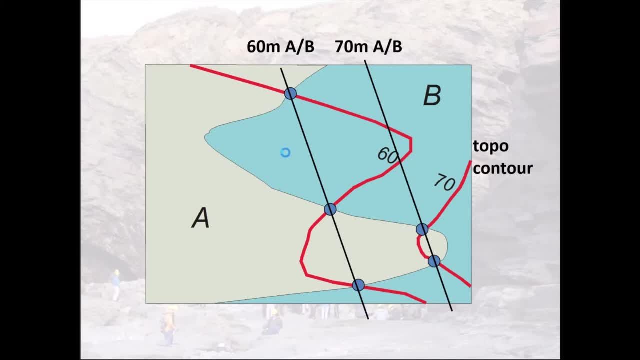 we haven't got any other structural contours. we can't. we can't find any other specific heights. we haven't got any other structural contours. we can't. we can't find any other specific heights. we haven't got any more um topography lines that intersect our contact. but maybe what we could do if we were. 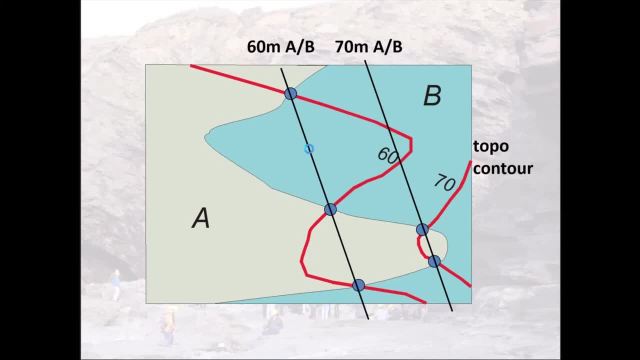 feeling fairly certain, we could extrapolate where the 50 meter contact would be. if we're on the 70 meter contact here and we're at the 60 meter contour there, if this plane is dipping at a constant angle, then we could interpret where the 50 meter structural contour would be. it would be. 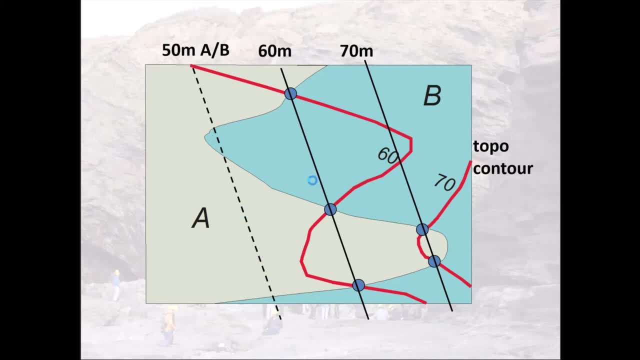 because it's a 10 meter structural contour. it would be a 10 meter structural contour. it would be a 10 meter interval from 70 to 60 and then 60 to 50. that spacing between the 70 and 60 meter structural contour would be the same as the spacing between the 60 and 50 meter structural contour. okay, we. 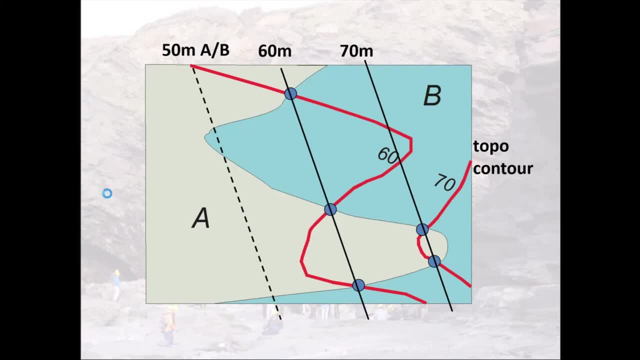 could continue this indefinitely either side of our map, to give us our 80 on our 40. but you can see, now that we've got these three structural contours which would allow us to figure out the direction of strike, of the of the contact, the direction of dip from high to low, of the contact from high to low, and if we had a scale, 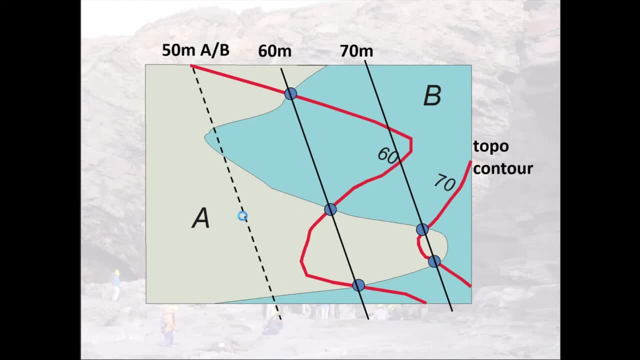 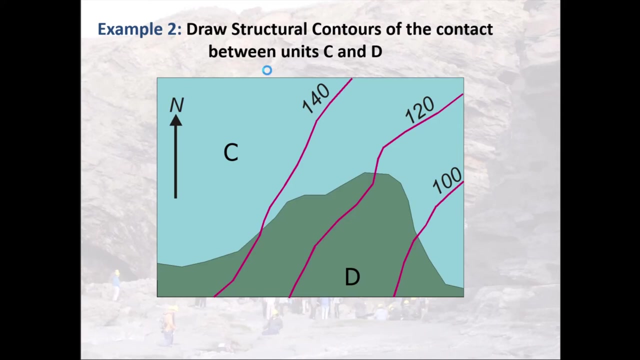 then maybe what we could do is figure out with some rudimentary trigonometry the angle of dip of that plane. okay, so that was a quite a nice example where we can, where we can basically just join the dots. but what if we had this sort of example where we've got another contact between two different rock types? 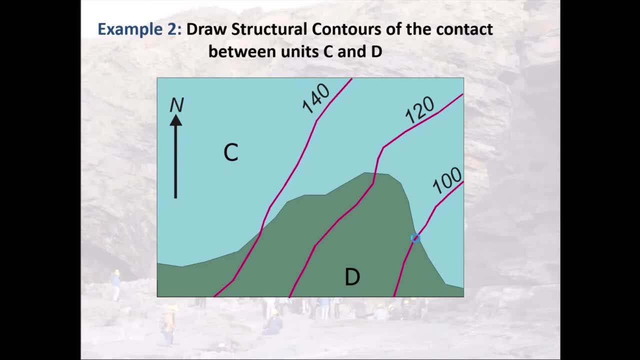 between c and d. this is our contact as it moves across the the ground surface and we can see where it intersects the topography in discrete points. but we haven't got anywhere where it intersects the same ground contour twice. how might we do that? take a few steps to see if we can. 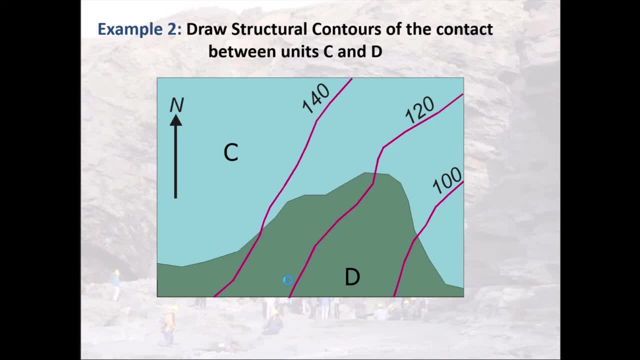 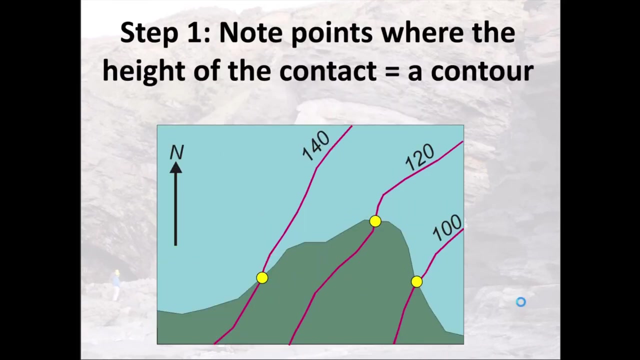 seconds. maybe pause the video to see if you can think of a way through this problem. okay, well, if you thought about that, maybe you've come to the answer. but let's, um, let's do it together. the first step in a situation like this is to know. 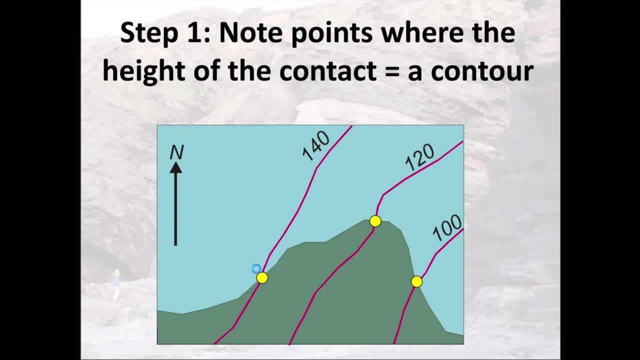 all of the points where you can define precisely what the height of the contact is. so here the height of the contact must be 100, 140, because it crosses the 140 topographic contour. here it's 120 and here it's 100. now, between this point, 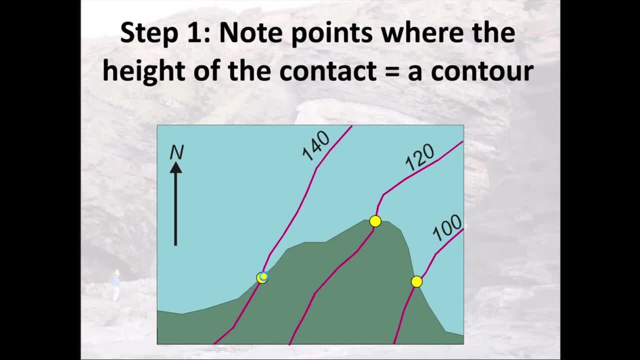 here at 100 and this point here at 140. you know that that plane must change: get through 120 meters. there's no way that you can go from a 140 meter contour to a 100 meter contour without going through the 120, so we must somewhere. 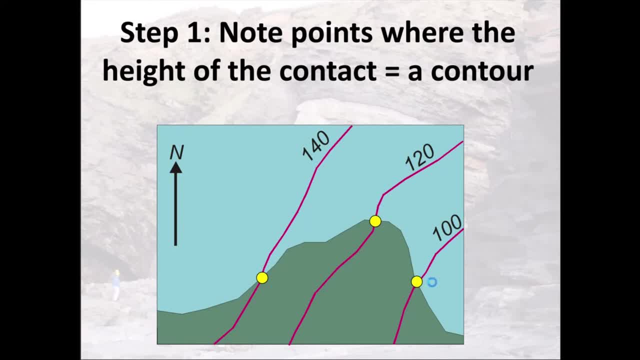 between these two points, we must cross the 120. now, if we're going to assume- and sometimes we don't, we shouldn't always assume, but if we're going to assume that this plane is, it has a uniform dip along it, it has a uniform dip along it. 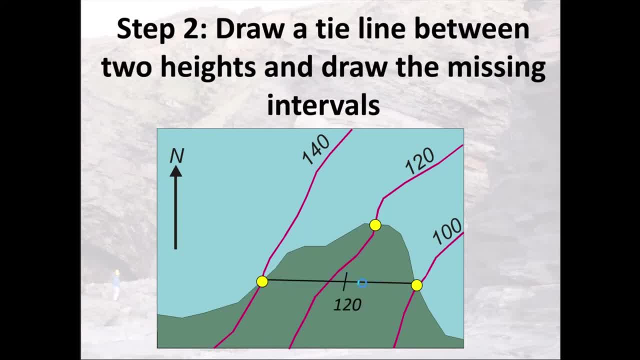 it has a uniform dip along it, then the point at which that plane hits, then the point at which that plane hits, then the point at which that plane hits, 120 is going to be halfway between 100. 120 is going to be halfway between 100. 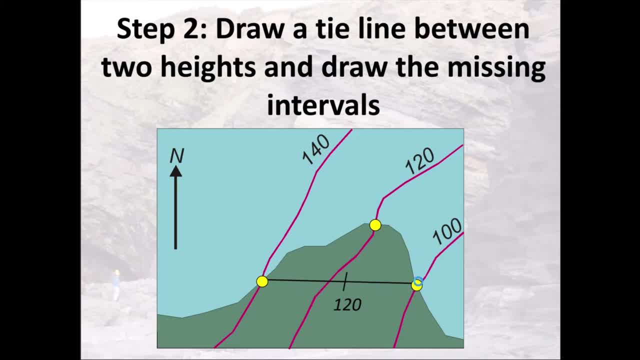 120 is going to be halfway between 100 and 140, so whatever this distance. and 140, so whatever this distance. and 140, so whatever this distance. between 140 and 110, is we just half it? between 140 and 110, is we just half it? 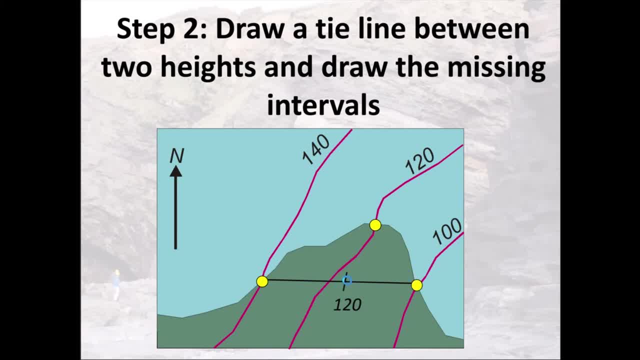 between 140 and 110, is we just half it and then mark on where this plane would, and then mark on where this plane would and then mark on where this plane would hit the 120 structural contour, now what. hit the 120 structural contour, now what? 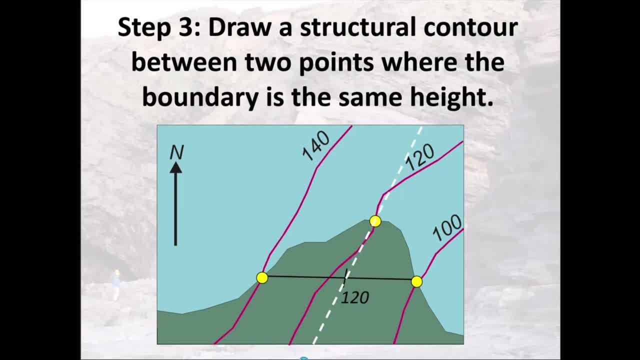 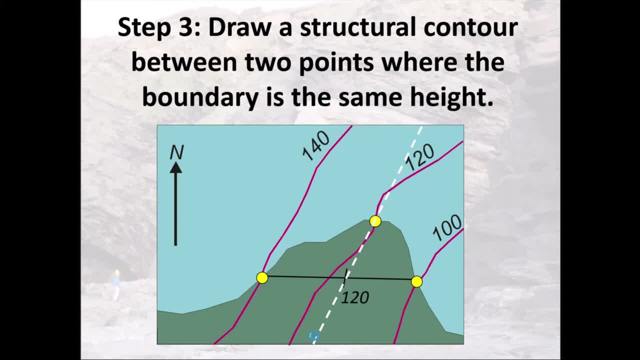 tie line we an interpreted and inferred structural contour that says that structural contour, that says that structural contour that says that everywhere along this line, the height of everywhere along this line, the height of everywhere along this line, the height of the contact between our two rock types, the contact between our two rock types, 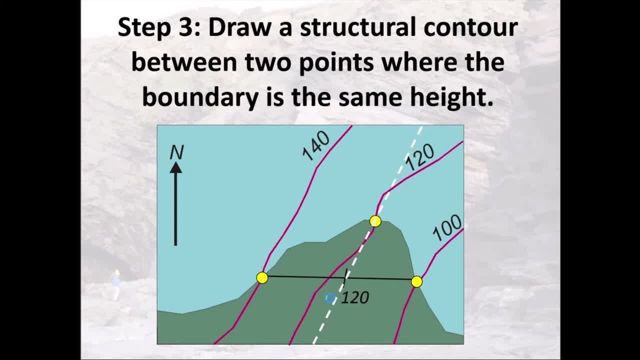 the contact between our two rock types, between the blue rock and the green rock, between the blue rock and the green rock, between the blue rock and the green rock, is going to be 120 once we've anchored. is going to be 120 once we've anchored. 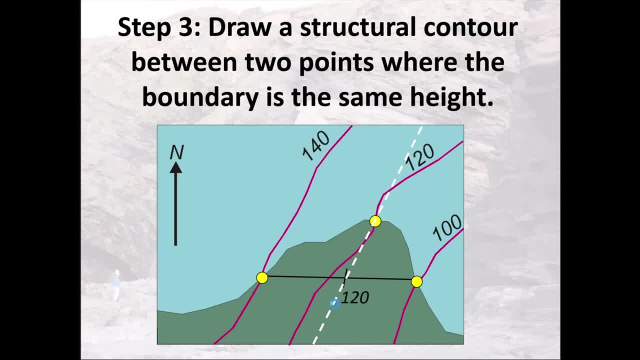 is going to be 120. once we've anchored ourselves with one of these structural ourselves, with one of these structural ourselves, with one of these structural contours, we can then infer the contours, we can then infer the contours, we can then infer the orientation of the others, and 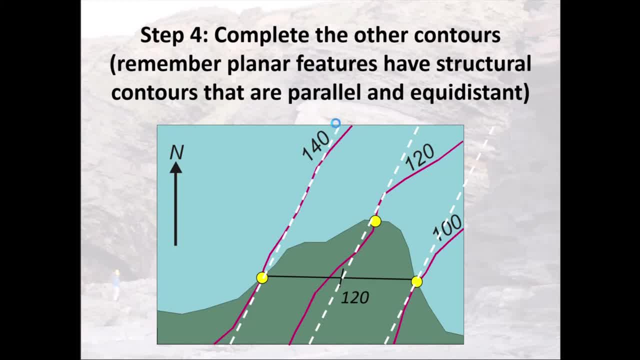 orientation of the others and orientation of the others. and again, if our plane is uniformly dipping, again, if our plane is uniformly dipping, again, if our plane is uniformly dipping, then each one of the structural contours, then each one of the structural contours, then each one of the structural contours is going to be parallel to each other. so 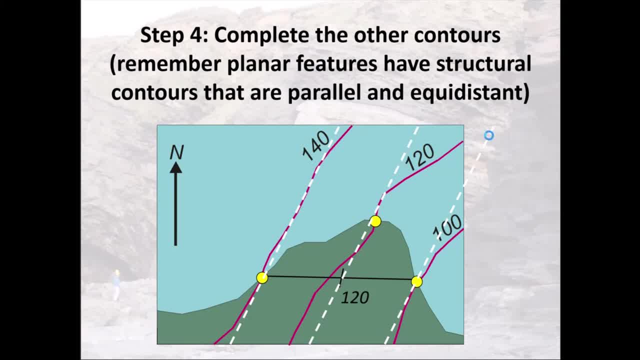 is going to be parallel to each other. so is going to be parallel to each other. so once we've got one in, we can then infer. once we've got one in, we can then infer. once we've got one in, we can then infer the positions of the others. I mean, the positions of the others. I mean the positions of the others. I mean that's all well and good, but at this, that's all well and good, but at this that's all well and good, but at this point you're probably asking me well if point. you're probably asking me, well if. 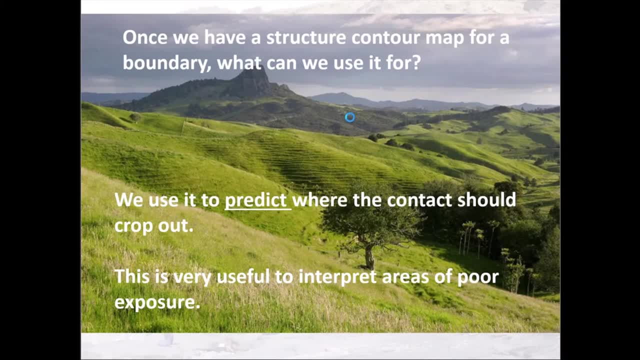 point. you're probably asking me: well, if I've already got a geological map, why am I've already got a geological map? why am I've already got a geological map? why am I bothering drawing structural contours? I bothering drawing structural contours, I bothering drawing structural contours. what is the point? I've already finished. 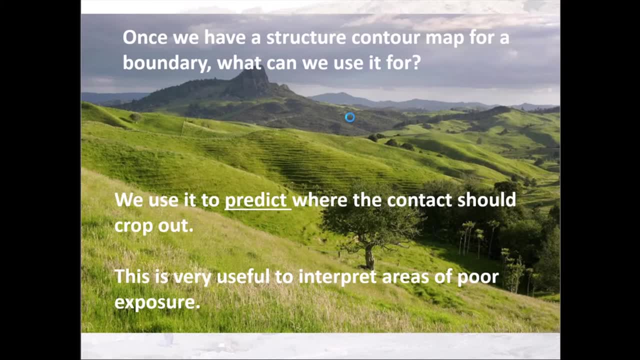 what is the point? I've already finished. what is the point? I've already finished the map. well, imagine that you've been the map. well, imagine that you've been the map. well, imagine that you've been able to. you're working in an area like able to. you're working in an area like 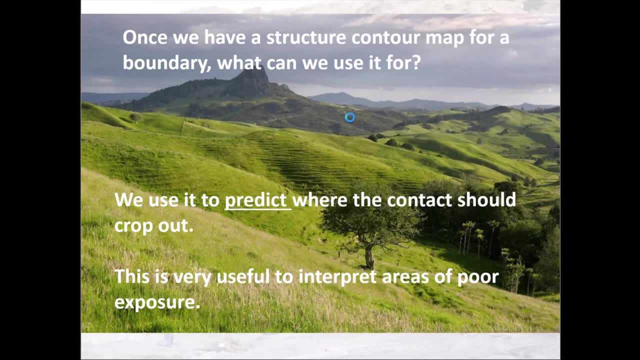 able to. you're working in an area like this where, largely, you've got very this, where, largely, you've got very this, where, largely, you've got very limited exposure. there's a couple of limited exposure, there's a couple of limited exposure. there's a couple of crags out in the distance, but the rest. 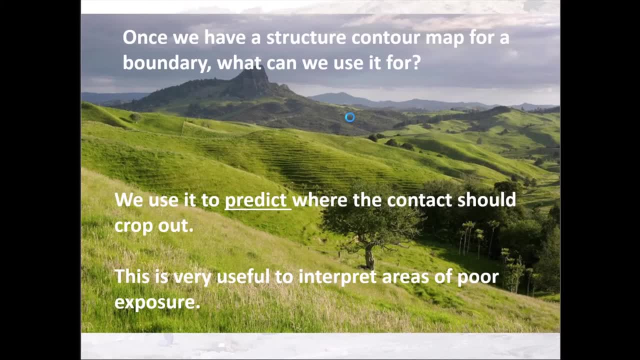 crags out in the distance. but the rest crags out in the distance. but the rest of the place, everything is covered by of the place, everything is covered by of the place, everything is covered by drift deposit. you can't see any real drift deposit. you can't see any real. 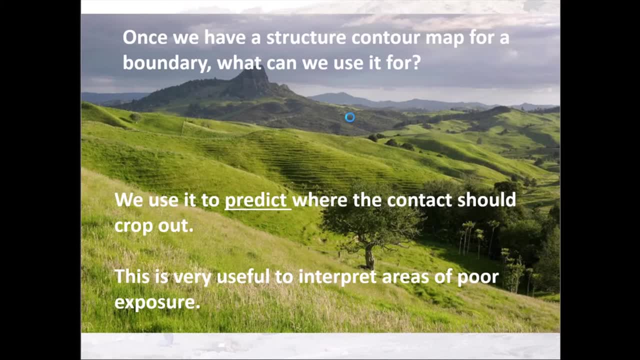 drift deposit. you can't see any real rocks. well, what you could actually do rocks well. what you could actually do rocks well. what you could actually do then is use a structural contour map. then is: use a structural contour map. then is use a structural contour map that you've been able to use or able to. 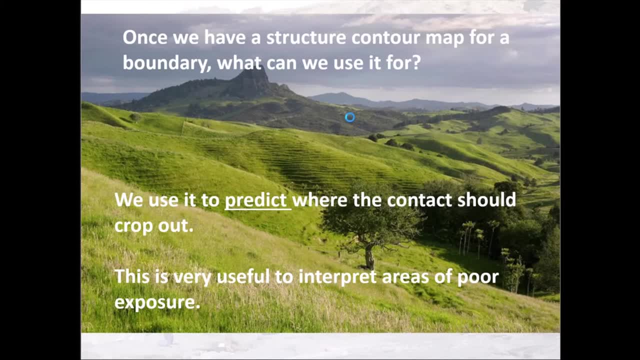 that you've been able to use or able to, that you've been able to use or able to produce from an area that does have a produce, from an area that does have a produce from an area that does have a bit of exposure, and use that to. 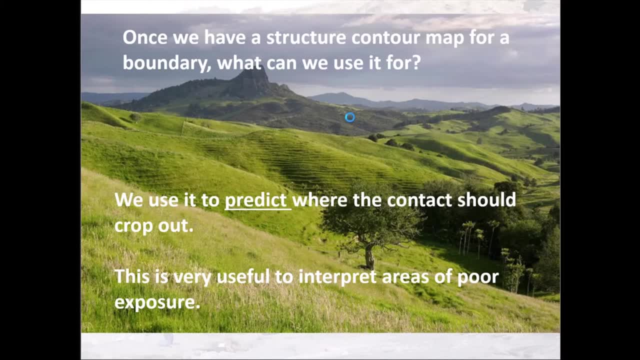 bit of exposure and use that to bit of exposure and use that to interpret where the geology would be in, interpret where the geology would be in interpret where the geology would be in areas of poor exposure. okay, so let's see areas of poor exposure. okay, so let's see. 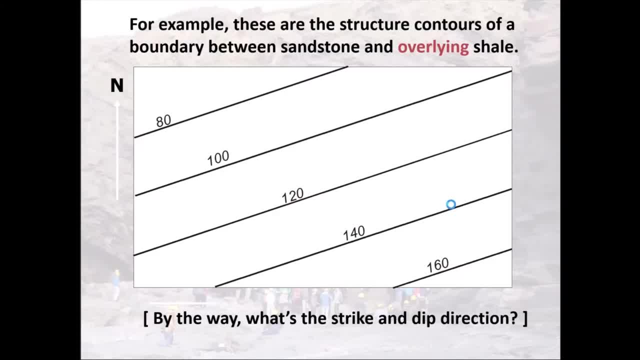 areas of poor exposure. okay, so let's see how we might do that with an example, how we might do that with an example, how we might do that with an example: okay, this is another map view. and this: okay, this is another map view. and this: okay, this is another map view and this set of structural contours shows you the 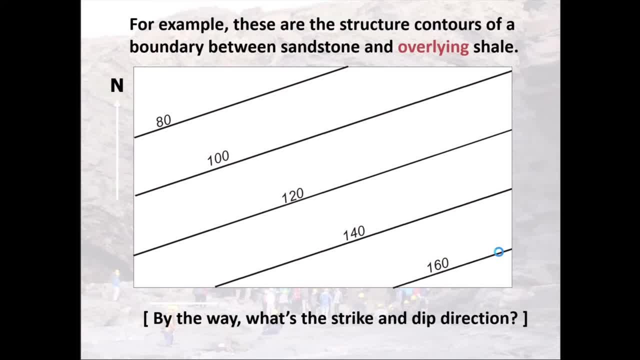 set of structural contours. shows you the set of structural contours. shows you the dip and strike. shows you the structural dip and strike. shows you the structural dip and strike. shows you the structural contours of a plane between sandstone. contours of a plane between sandstone. contours of a plane between sandstone and an overlying shale. so we've got the. 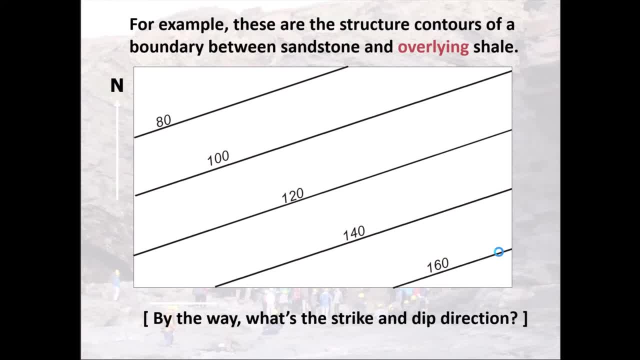 and an overlying shale, so we've got the and an overlying shale, so we've got the sedimentary contact, the plane of which sedimentary contact, the plane of which sedimentary contact, the plane of which we've represented with these structural, we've represented with these structural. 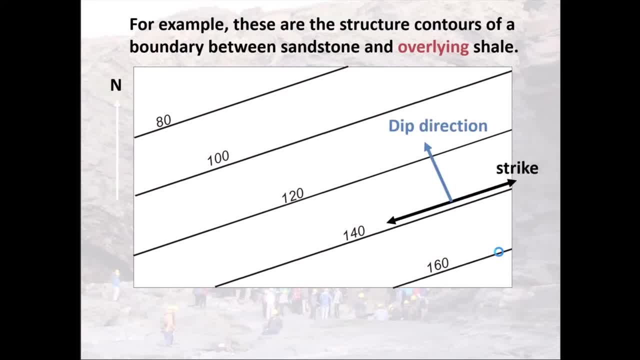 we've represented with these structural contours again just as an aside. our contours again just as an aside. our contours again just as an aside. our strike is going to be parallel to the strike, is going to be parallel to the strike, is going to be parallel to the structural contours and our dip. 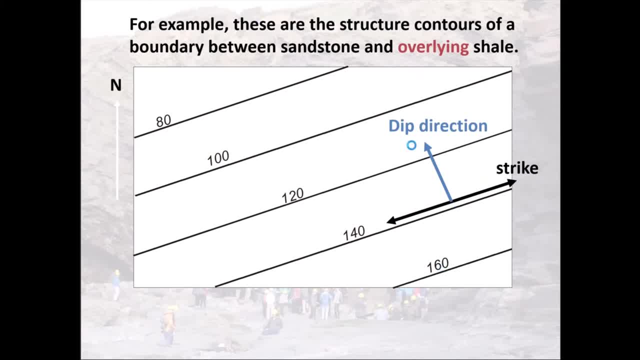 structural contours and our dip structural contours and our dip direction is going to go from high to direction. is going to go from high to direction. is going to go from high to low perpendicular to those contours- okay, low perpendicular to those contours- okay, low perpendicular to those contours- okay, then what we're going to do is overlay. 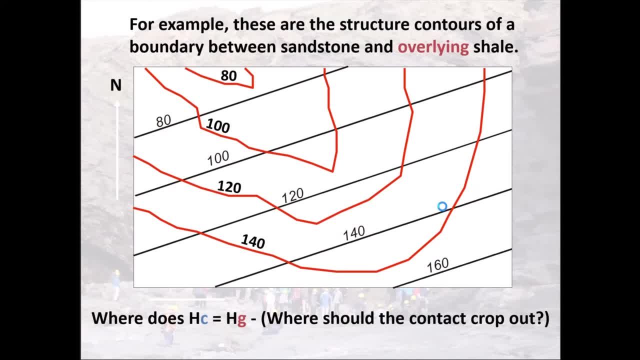 then what we're going to do is overlay. then what we're going to do is overlay our topography, our topographic contours, our topography, our topographic contours, our topography, our topographic contours, our red lines on to our structural, our red lines on to our structural. 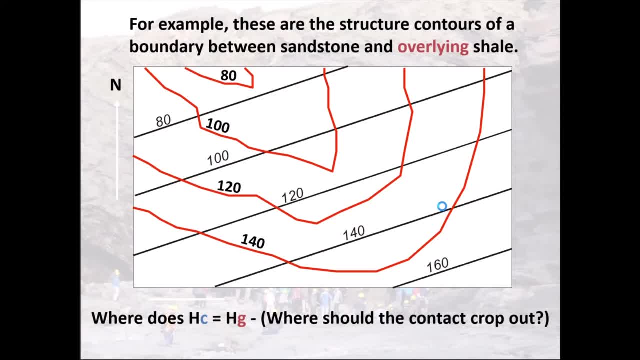 our red lines on to our structural contour map. now you guys remember from contour map. now you guys remember from contour map. now you guys remember from the previous slides that wherever the the previous slides, that wherever the the previous slides, that wherever the height of the contact equals the height, 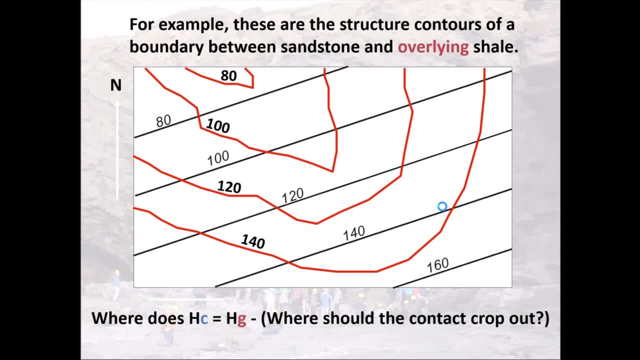 height of the contact equals the height. height of the contact equals the height of the ground. that's where we should see of the ground. that's where we should see of the ground. that's where we should see the contact on the surface. that's where the contact on the surface, that's where 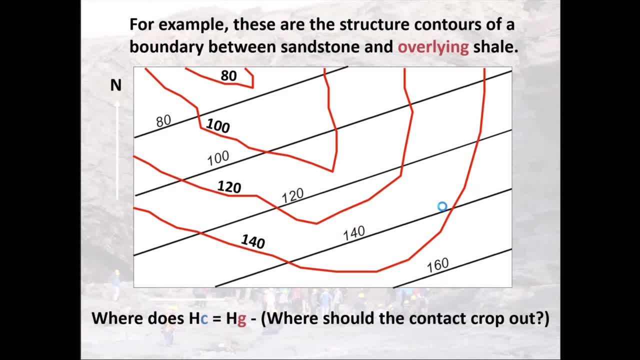 the contact on the surface. that's where the contact between the sandstone and the, the contact between the sandstone and the, the contact between the sandstone and the overlying shale. that's where it will overlying shale, that's where it will overlying shale, that's where it will crop out on the map. so what we need to do, 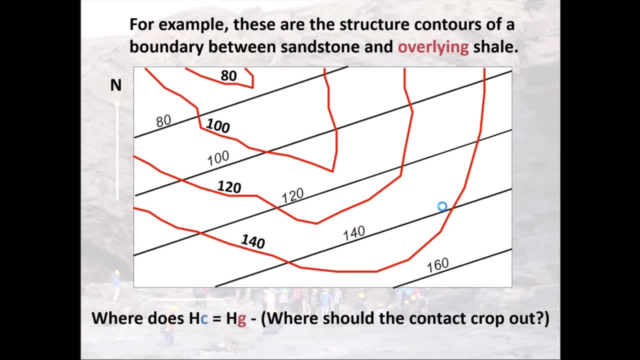 crop out on the map. so what we need to do crop out on the map. so what we need to do is find everywhere where our structural is find everywhere where our structural is find everywhere where our structural contours equal the height of our ground. contours equal the height of our ground. 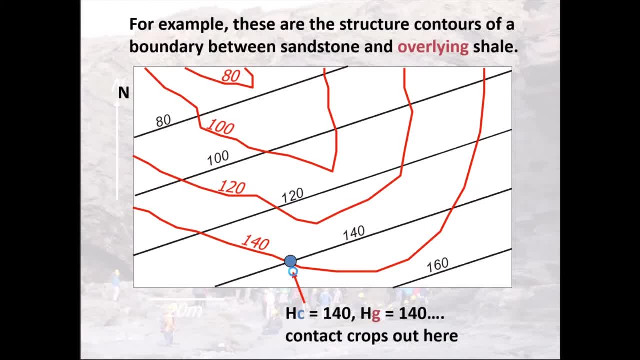 contours equal the height of our ground contours. so we've got one here there, the contours. so we've got one here there, the contours. so we've got one here there. the height of the ground is 140, and the height of the ground is 140 and the 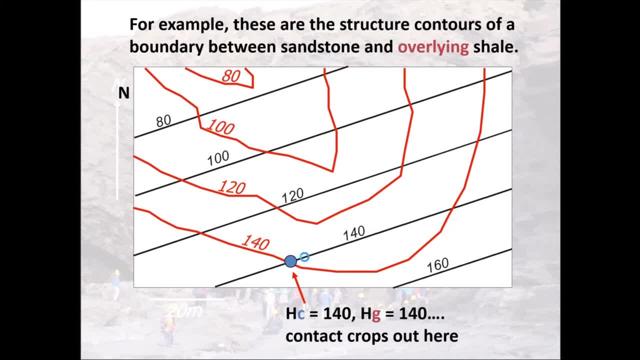 height of the ground is 140 and the height of the plane is 140. so at that height of the plane is 140. so at that height of the plane is 140. so at that point where they intersect, that's where. point where they intersect, that's where. 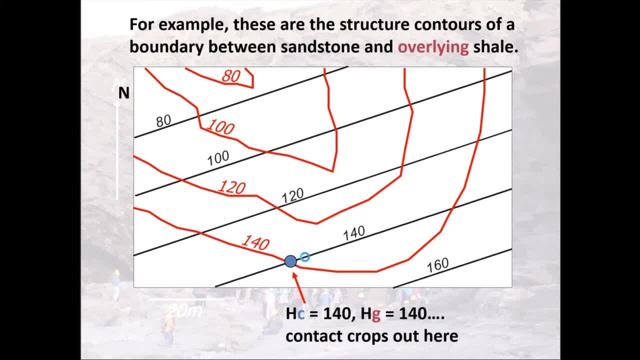 point where they intersect. that's where the contact would crop out on the ground. the contact would crop out on the ground. the contact would crop out on the ground surface. where else can we find it well surface? where else can we find it well surface? where else can we find it well? I've got 120, 120, we've got 100, 100, the. I've got 120, 120. we've got 100, 100, the. I've got 120, 120. we've got 100, 100, the 80 and the 80, they don't intersect. so 80 and the 80, they don't intersect. so 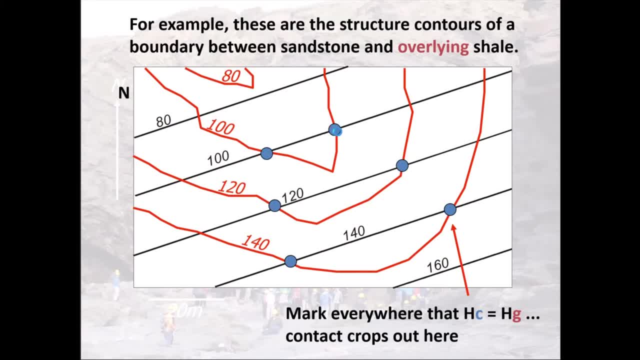 80 and the 80, they don't intersect. so it's not going to hit there, it hits our. it's not going to hit there, it hits our. it's not going to hit there, it hits our. hundred, 120, 140 again. so we've marked. 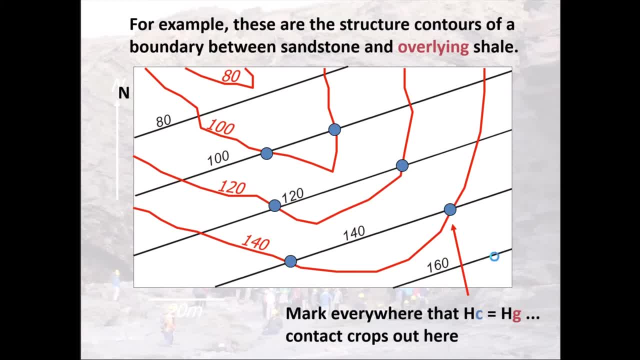 hundred 120, 140 again. so we've marked hundred 120, 140 again. so we've marked everywhere that the height of the everywhere, that the height of the everywhere, that the height of the contact equals the height of the ground, so we've got these series of points and 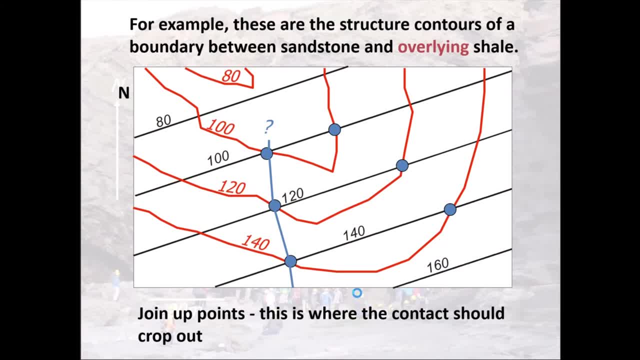 so we've got these series of points, and so we've got these series of points, and then you guys have probably guessed it, then you guys have probably guessed it, then you guys have probably guessed it in order to work out the run of the. in order to work out the run of the. 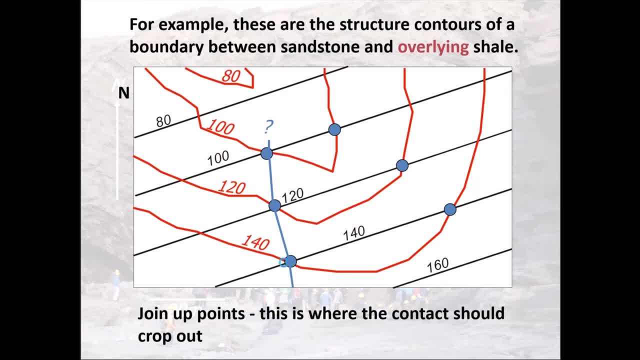 in order to work out the run of the contact, we simply join up these points where each one of them is an, where each one of them is an, where each one of them is an intersection between the topographic intersection, between the topographic intersection between the topographic contour and our structural contour. so 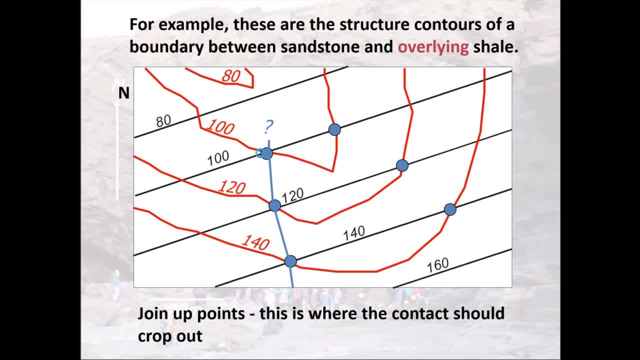 contour and our structural contour. so contour and our structural contour. so here at 140, we can join up to our 120. here at 140, we can join up to our 120. here at 140, we can join up to our 120, we can join up to our 100. at this point we 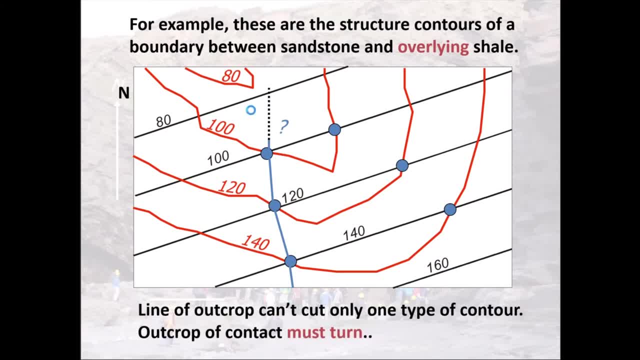 we can join up to our 100 at this point. we we can join up to our 100 at this point. we can't just continue up to our 80, can't just continue up to our 80, can't just continue up to our 80 because, if you look back at the map, our 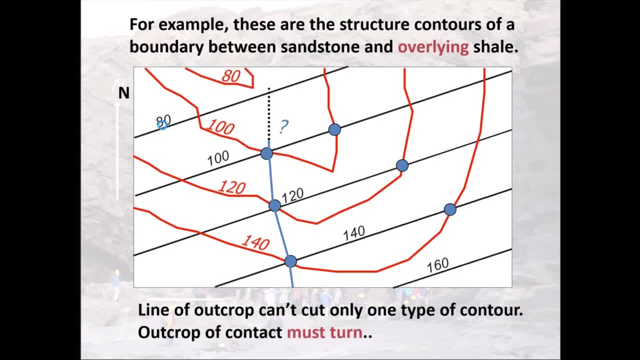 because if you look back at the map, our, because if you look back at the map, our 80 topographic contour does not 80 topographic contour, does not 80 topographic contour does not intersect our 80 ground height, so intersect our 80 ground height. so 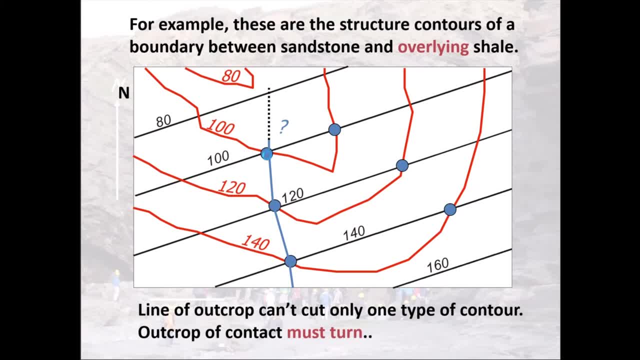 intersect our 80 ground height. so because there's no intersection, then our, because there's no intersection, then our, because there's no intersection, then our stratigraphic contact between our two stratigraphic contact between our two, stratigraphic contact between our two rock types. it cannot progress that way. 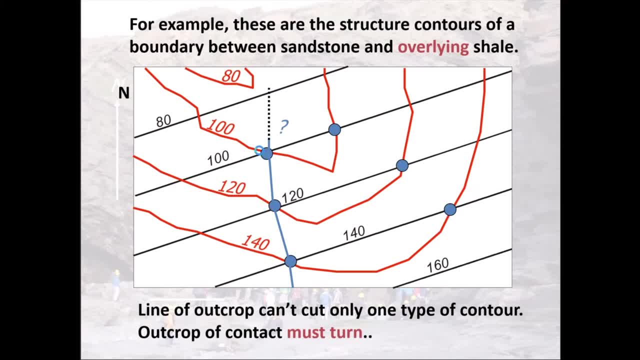 instead, the run of the contact must turn. instead, the run of the contact must turn. instead, the run of the contact must turn to join up with the other intersections, to join up with the other intersections, to join up with the other intersections of our structural contours and of our structural contours. and 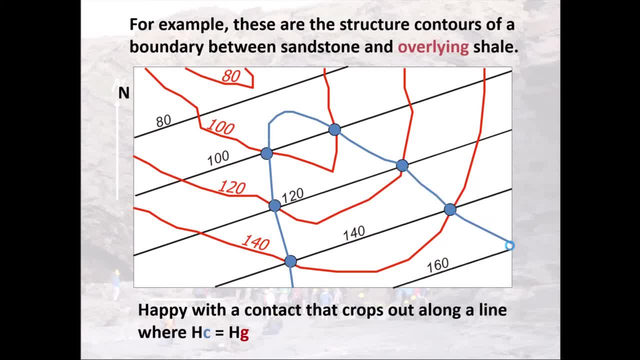 of our structural contours and topographic contours. okay, I've just topographic contours. okay, I've just topographic contours. okay, I've just continued it out this way. because you continued it out this way, because you continued it out this way because you know it, you know PowerPoint and I didn't 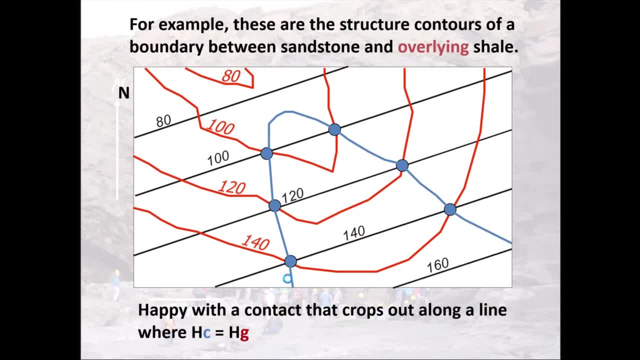 know it. you know PowerPoint and I didn't know it. you know PowerPoint and I didn't have a 160 topographic line. okay, so have a 160 topographic line, okay. so have a 160 topographic line, okay. so here we've got our contact between our two. 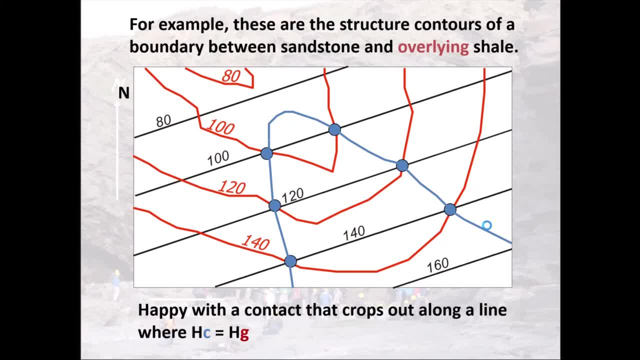 here we've got our contact between our two. here we've got our contact between our two rock units, between our sandstone and rock units, between our sandstone and rock units, between our sandstone and our overlying shale. great. so this is the boundary between great. so this is the boundary between. 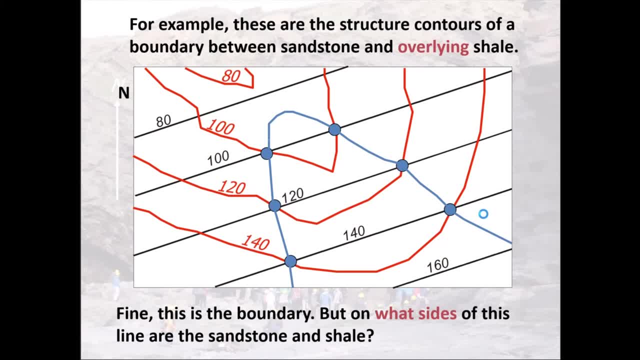 great. so this is the boundary between our rock unit. but now we need to ask our rock unit. but now we need to ask our rock unit. but now we need to ask ourselves: okay, which side of the ourselves, okay, which side of the ourselves, okay, which side of the boundary would our sandstone be? 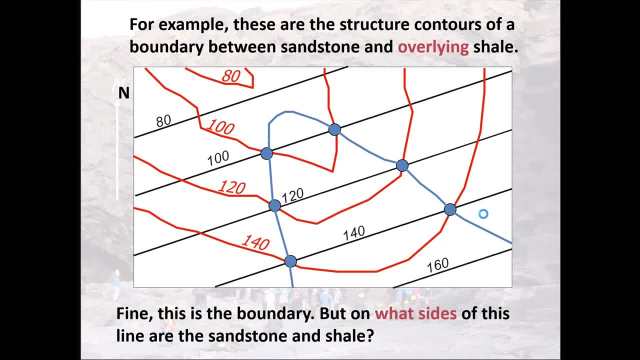 boundary would our sandstone be? boundary would our sandstone be, and which side of the boundary would our and which side of the boundary would our and which side of the boundary would our shale be? take a minute to think about that, this. take a minute to think about that, this. 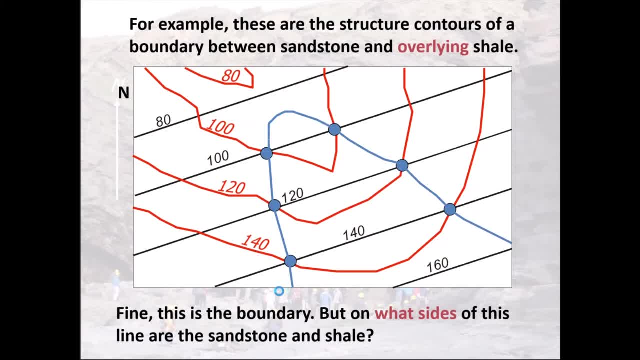 take a minute to think about that. this is our contact. so we know that there is. is our contact. so we know that there is. is our contact. so we know that there is sensor and share leader side of it, but sensor and share leader side of it, but. 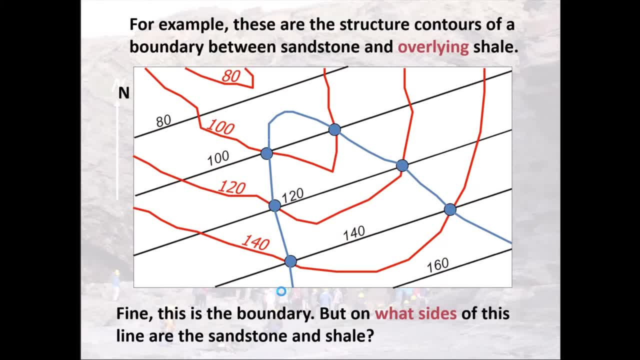 sensor and share leader side of it. but which side is which? okay, well, you can think about this. okay, well, you can think about this. okay, well, you can think about this. way. this is the way that makes most sense. way, this is the way that makes most sense. 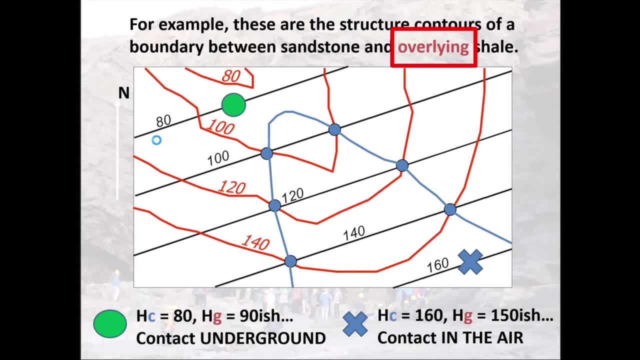 way. this is the way that makes most sense to me. if we were to take two points to me, if we were to take two points to me, if we were to take two points either side of the contact, let's start. either side of the contact, let's start. 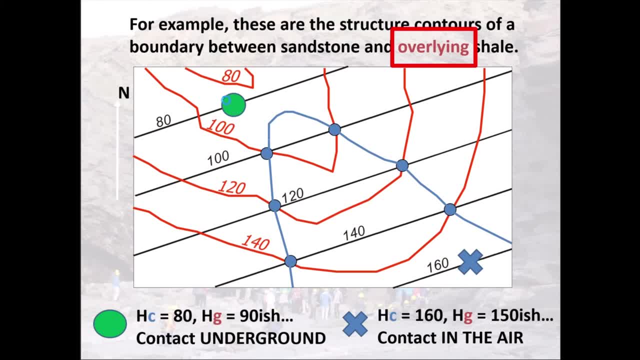 either side of the contact. let's start with this one here. the ground height is with this one here. the ground height is with this one. here the ground height is about 90 ish. we're halfway between the about 90 ish. we're halfway between the. 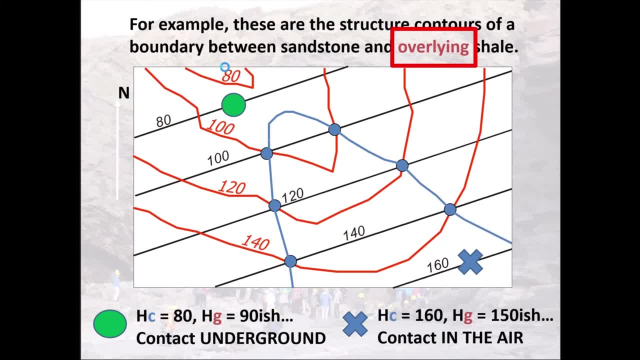 about 90 ish. we're halfway between the 100 and the 80 topographic contour, but 100 and the 80 topographic contour, but 100 and the 80 topographic contour, but the height of the contact is 80, so here, the height of the contact is 80, so here. 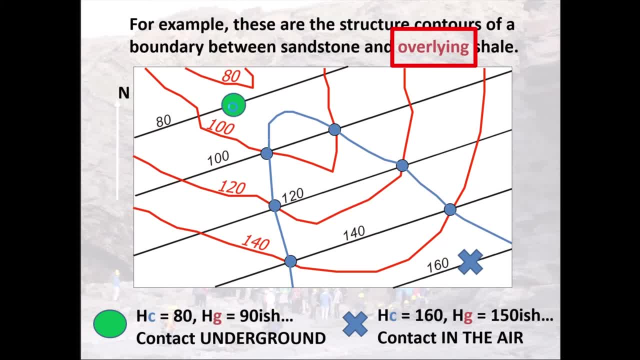 the height of the contact is 80. so here the height of the ground is higher than. the height of the ground is higher than. the height of the ground is higher than the. the height of the ground is higher the. the height of the ground is higher the. the height of the ground is higher than the height of the contact over here. 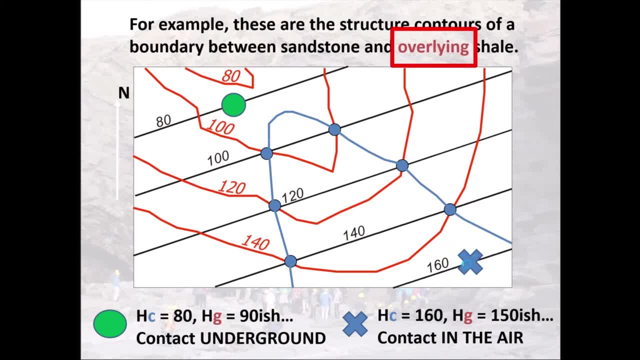 than the height of the contact over here, than the height of the contact over here. the height of the contact is 160 and the the height of the contact is 160 and the. the height of the contact is 160 and the height of the ground is somewhere. 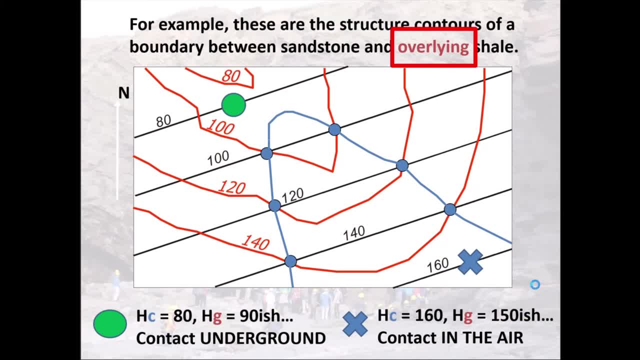 height of the ground is somewhere. height of the ground is somewhere between 140 here and wherever 160 would between 140 here and wherever 160 would between 140 here and wherever 160 would be over here. so here the height of the be over here. so here the height of the. 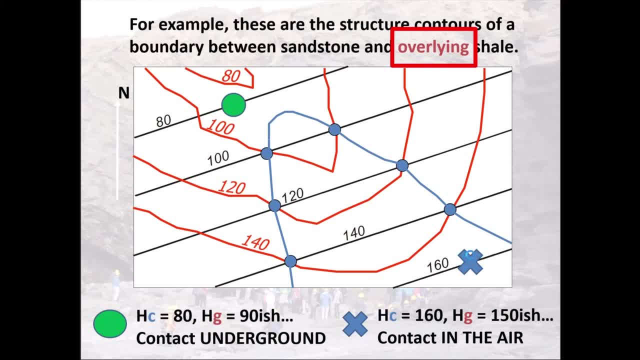 be over here. so here the height of the contact is higher than the height of the contact is higher than the height of the contact is higher than the height of the ground. so if we were to draw just a ground, so if we were to draw just a, 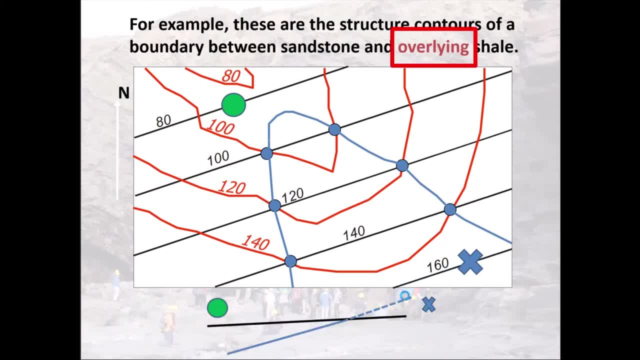 ground. so if we were to draw just a schematic cross-section through that over schematic cross-section through that, over schematic cross-section through that, over here, our blue cross, the height of the here, our blue cross, the height of the here, our blue cross, the height of the contact, is higher than the height of the. 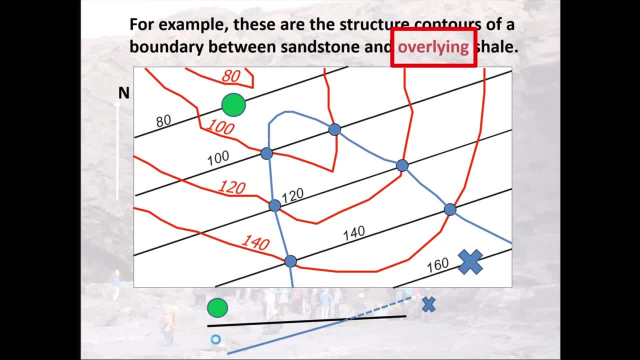 contact is higher than the height of the contact is higher than the height of the ground, and over here our green dot, the ground, and over here our green dot, the ground, and over here our green dot, the height of the contact is lower than the height of the contact is lower than the. 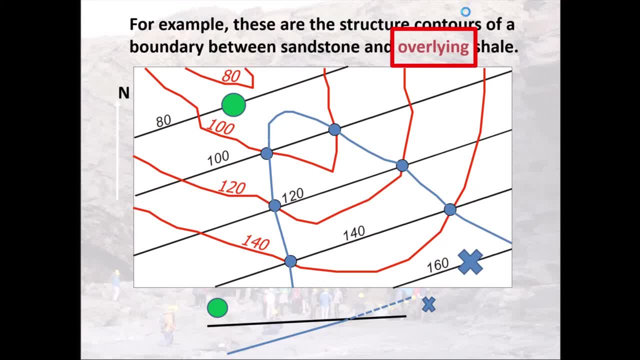 height of the contact is lower than the height of the ground. so, for our purposes, height of the ground. so, for our purposes, height of the ground. so, for our purposes, where we've got this stratigraphic, where we've got this stratigraphic, where we've got this stratigraphic relationship between a sandstone and an? 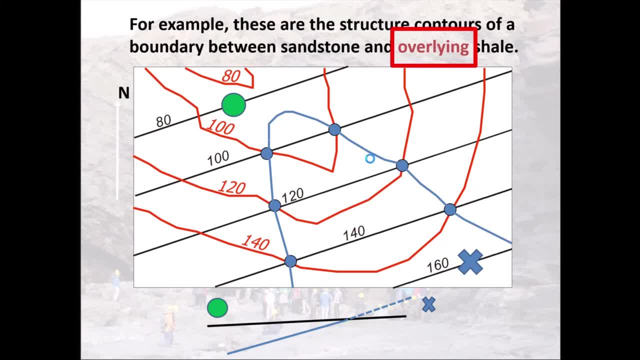 relationship between a sandstone and an relationship between a sandstone and an overlying shale, then the only way that overlying shale, then the only way that overlying shale, then the only way that could work in our schematic cross-section could work in our schematic cross-section. 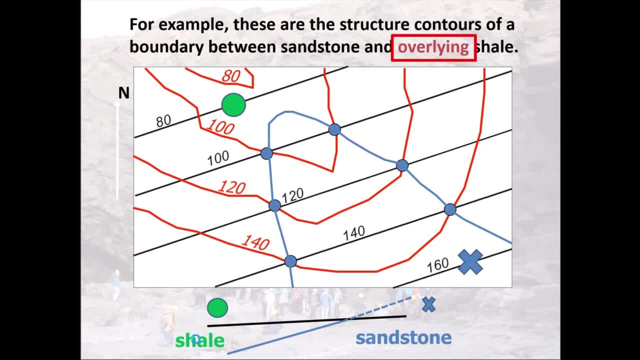 could work in our schematic cross-section: is if this side is our sandstone and is if this side is our sandstone and is if this side is our sandstone and this side is our shale. so once we figure, this side is our shale. so once we figure, 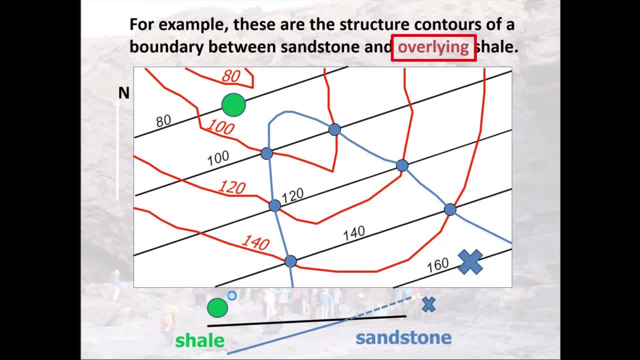 this side is our shale. so once we figure that out, once we've got the that out, once we've got the that out, once we've got the understanding of our outcrop contact and understanding of our outcrop contact and understanding of our outcrop contact, and we know which side of the outcrop, both 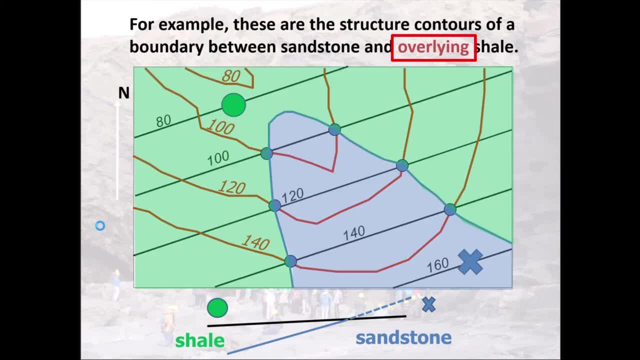 we know which side of the outcrop both. we know which side of the outcrop both of our units are cropping out. we can of our units are cropping out. we can of our units are cropping out. we can then finish our map showing the. then finish our map showing the. 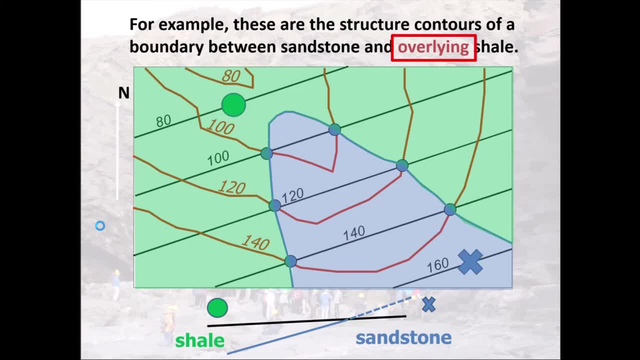 then finish our map showing the distribution of our two rock types. if distribution of our two rock types. if distribution of our two rock types. if you want to replay that a few times, you want to replay that a few times. you want to replay that a few times. that's fine. that one of the things about 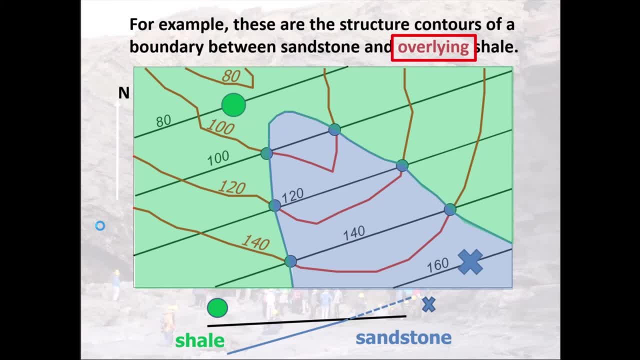 that's fine, that one of the things about that's fine, that one of the things about this geological visualization is: if this geological visualization is, if this geological visualization is, if you've, if you've got a predisposition to you've, if you've got a predisposition to think about things in three dimensions. 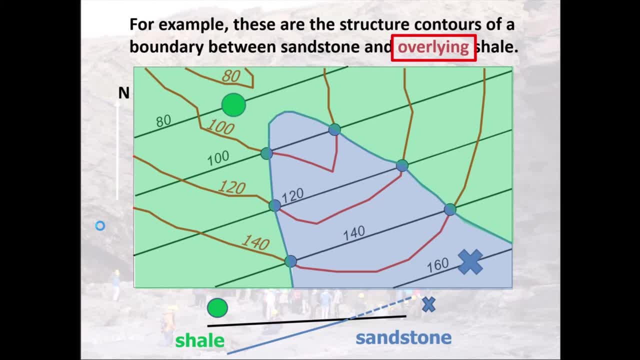 think about things in three dimensions. think about things in three dimensions. you probably pick this up quite quickly. you probably pick this up quite quickly. you probably pick this up quite quickly. but if you haven't, then that's why we. but if you haven't, then that's why we. 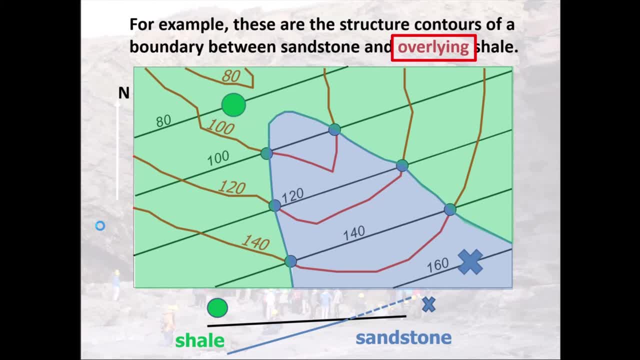 but if you haven't, then that's why we record these things for you, so you can record these things for you. so you can record these things for you, so you can take your time with it and get in touch. take your time with it and get in touch. 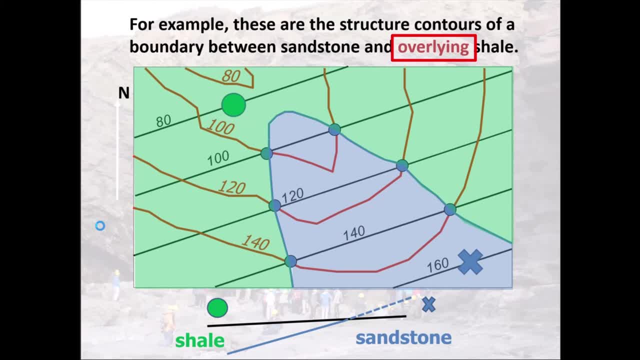 take your time with it and get in touch with me otherwise now, briefly, what I with me otherwise, now briefly, what I with me otherwise now briefly, what I want to show you as we as we finish is want to show you as we as we finish, is want to show you as we as we finish, is how we can use these structural contours. 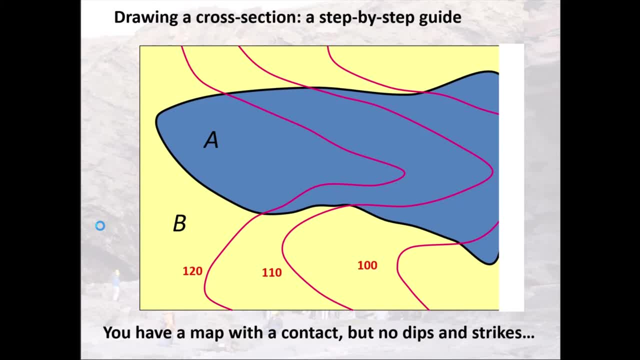 how we can use these structural contours, how we can use these structural contours to help build a cross-section like an. to help build a cross-section like an. to help build a cross-section like an actual one, not just this sort of you know- actual one, not just this sort of you know. 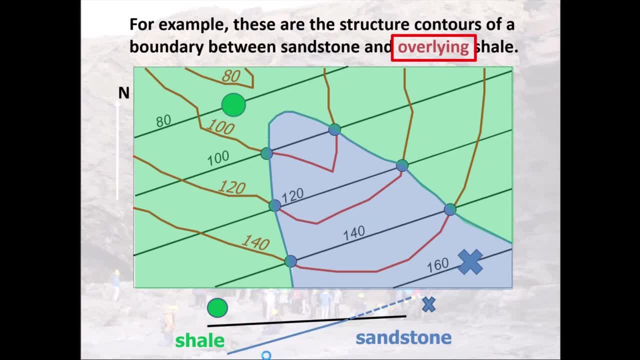 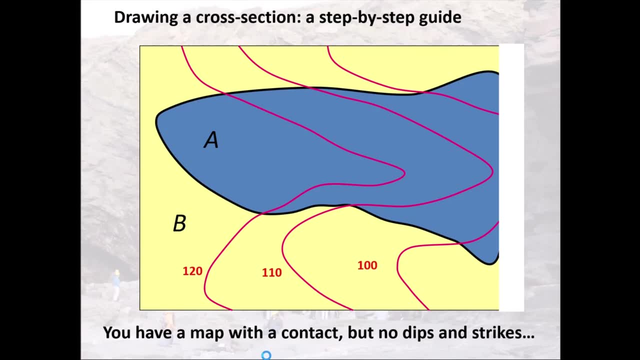 actual one, not just this sort of, you know, handy little thought experiment and handy little thought experiment and handy little thought experiment and conceptual model, how we actually use conceptual model, how we actually use conceptual model, how we actually use them to build a real cross-section, so them to build a real cross-section. so 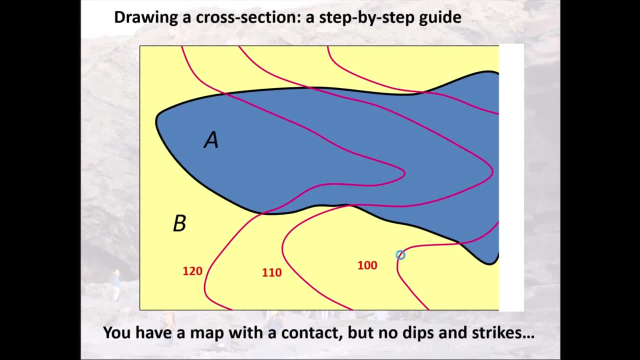 them to build a real cross-section. so let's take this example. this is a. let's take this example. this is a. let's take this example. this is a rudimentary geological map. we've got two rudimentary geological map. we've got two rudimentary geological map. we've got two rock units. we've got this B, and then 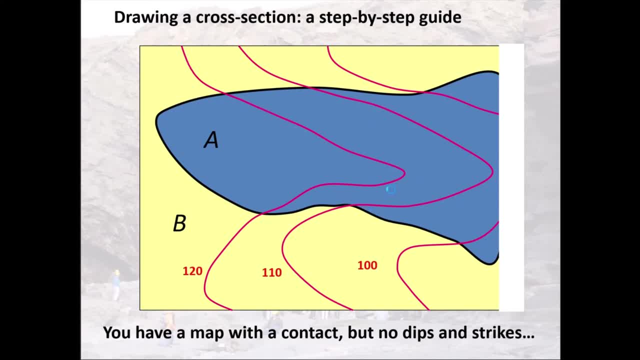 rock units, we've got this B, and then rock units, we've got this B, and then we've got this a and we've got some red. we've got this a and we've got some red. we've got this a and we've got some red. topographic contours: we don't have any. 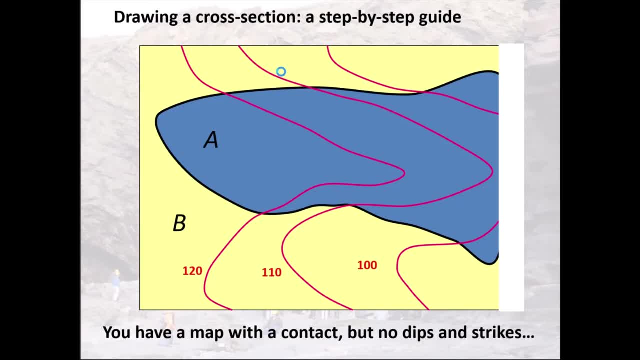 topographic contours? we don't have any topographic contours. we don't have any dips and strikes, so we can't just use an dips and strikes. so we can't just use an dips and strikes. so we can't just use an angle from the map and draw it on our 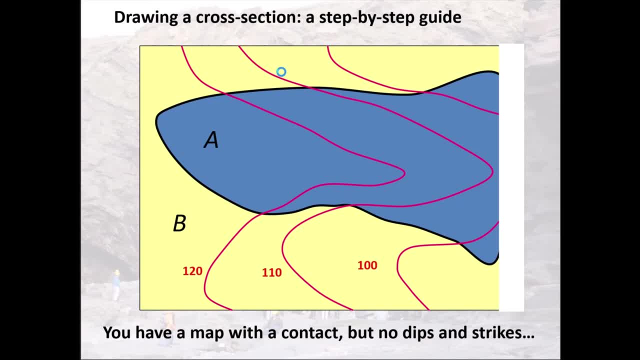 angle from the map and draw it on our angle from the map and draw it on our cross-section. so instead we're going to cross-section. so instead we're going to cross-section. so instead we're going to have to figure out what the dip is using. 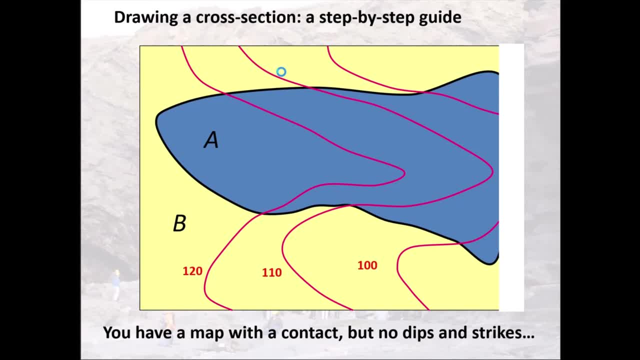 have to figure out what the dip is using, have to figure out what the dip is using- structural contours. so what we need to structural contours, so what we need to structural contours. so what we need to do is find specific points where we know. do is find specific points where we know. 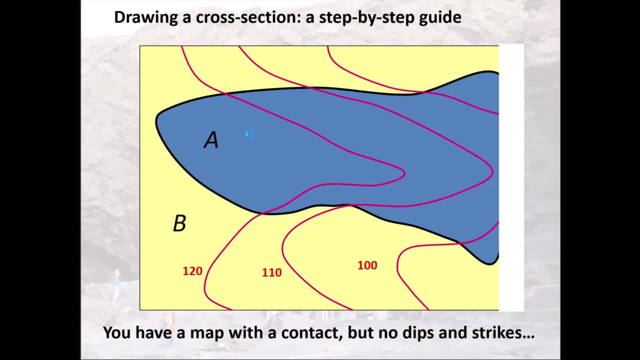 do is find specific points where we know the height of the contact, for example, the height of the contact. for example, the height of the contact, for example, here and here. the contact on our map: the here and here. the contact on our map: the here and here. the contact on our map. the geological contact intersects the 120. 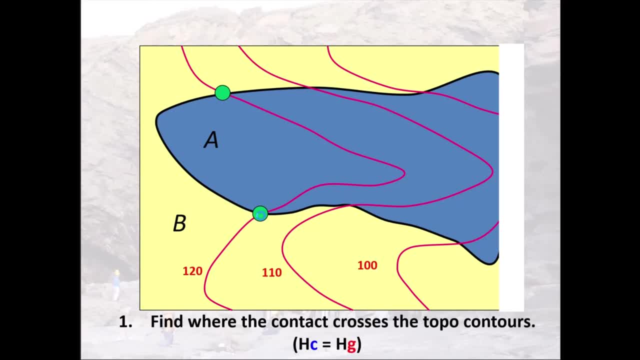 geological contact intersects the 120 geological contact intersects the 120 structural contour. sorry, it intersects structural contour. sorry, it intersects structural contour. sorry, it intersects the 120 topographic contour. so we can the 120 topographic contour, so we can the 120 topographic contour. so we can link those two points and draw our 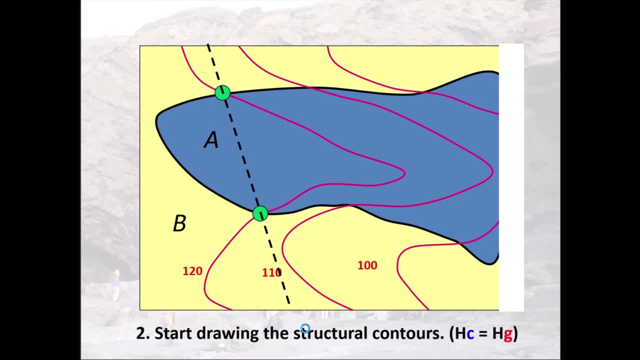 link those two points and draw our link, those two points and draw our selves: a 120 meter structural contour, selves a 120 meter structural contour. selves a 120 meter structural contour for the contact here and here it for the contact here and here it for the contact here, and here it intersects the 110 topographic contour. 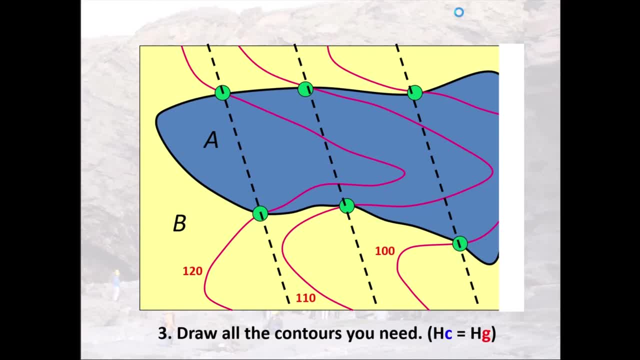 intersects the 110 topographic contour, intersects the 110 topographic contour and here and here it intersects the 100 and here and here it intersects the 100 and here and here it intersects the 100. topographic contours- we've got this set. topographic contours. we've got this set. 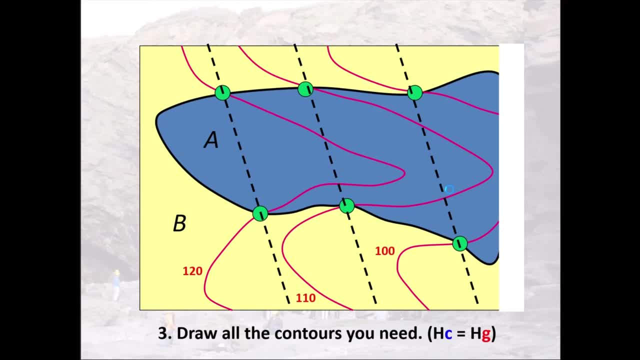 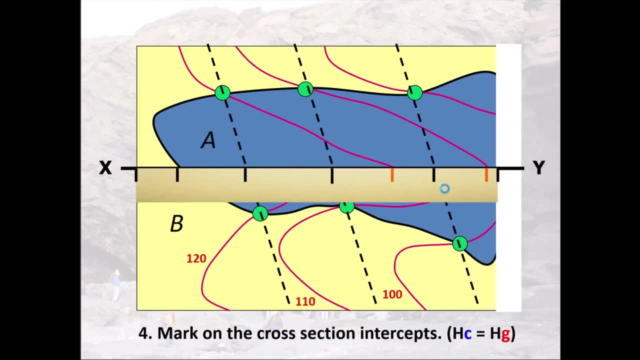 topographic contours. we've got this set of structural contours which we can then of structural contours which we can then of structural contours which we can then use to build us a cross-section use to build us a cross-section, use to build us a cross-section. okay, so, just like we did in the previous, 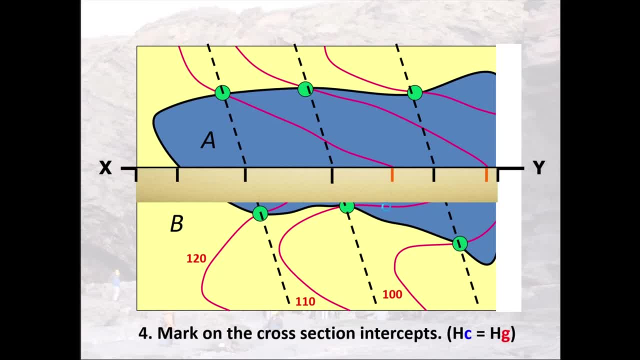 okay, so, just like we did in the previous. okay, so, just like we did in the previous. examples from previous weeks. we'd use examples from previous weeks. we'd use examples from previous weeks. we'd use our strip of paper and in red, I have our strip of paper and in red I have. 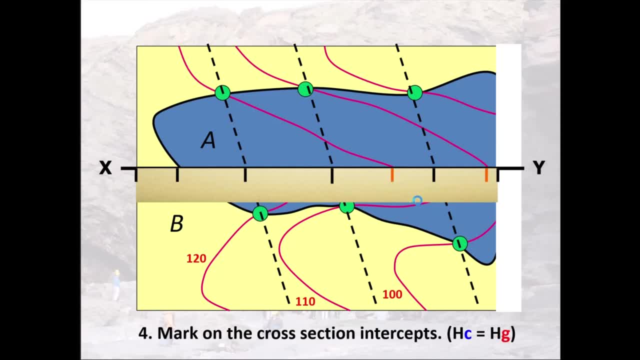 our strip of paper and in red, I have marked on the points at which you the marked on the points at which you the marked on the points at which you the cross-section crosses topographic cross-section crosses topographic cross-section crosses topographic contours. so this topographic contour, 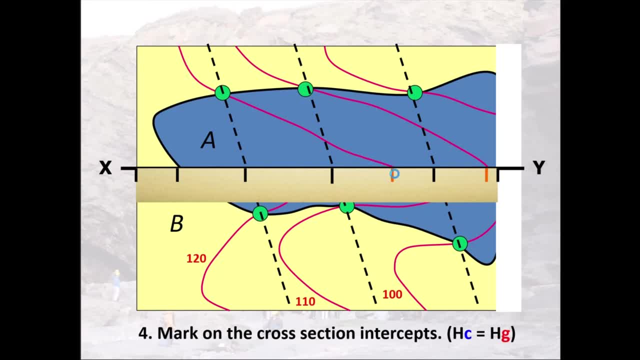 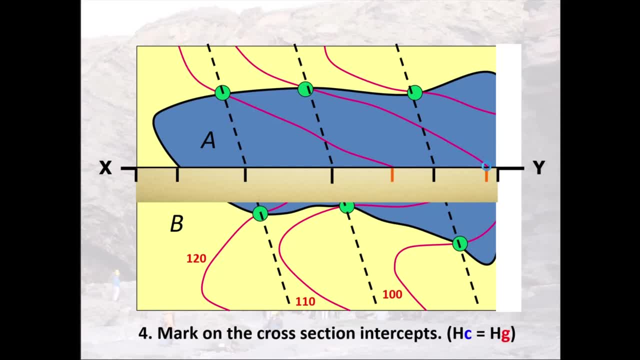 this topographic contour is 110, and this topographic contour is 110 and intersects our cross-section there and intersects our cross-section there and intersects our cross-section there, and then what I've also marked on is all of then. what I've also marked on is all of. 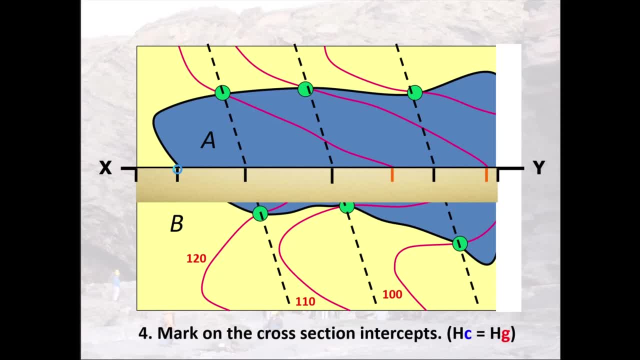 then, what I've also marked on is all of the points at which I know the height of the points at which I know the height of the points at which I know the height of the contact between A and B. I know the, the contact between A and B. I know the. 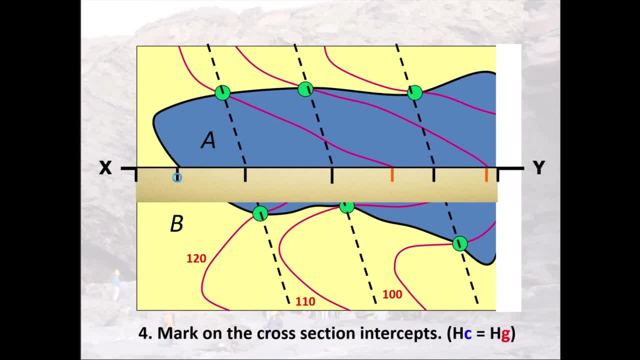 the contact between A and B. I know the height of the contact A and B is. height of the contact A and B is height of the contact A and B is whatever the ground height is. I know that, whatever the ground height is, I know that whatever the ground height is, I know that the height of the contact between A and B 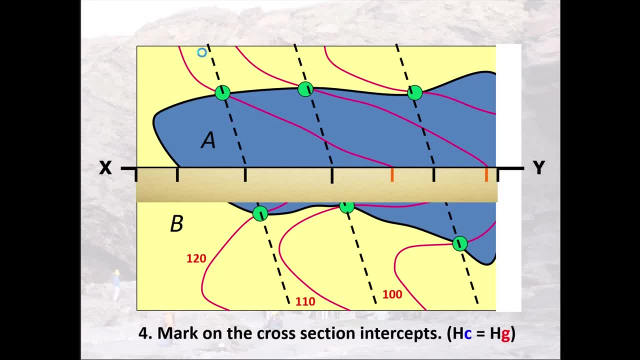 the height of the contact between A and B is 100 and 10. because that's where the 100 and 10, because that's where the 100 and 10, because that's where the structural contour intersects our structural contour intersects our structural contour intersects our cross-section. I know that the height of 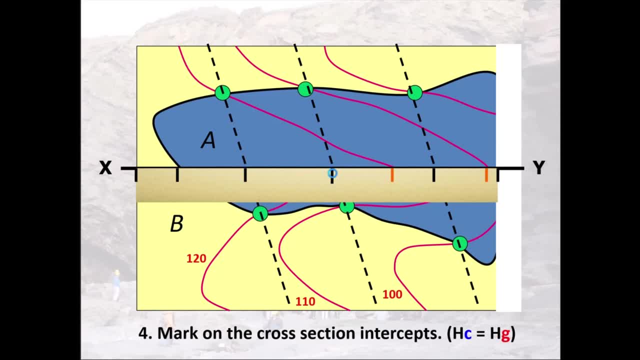 cross-section. I know that the height of cross-section, I know that the height of the contact there is sorry, this is 110. the contact there is sorry, this is 110. the contact there is sorry, this is 110, that's 120. and I know the height of the. 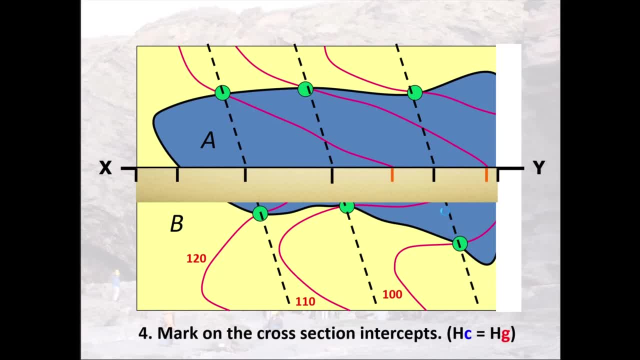 that's 120 and I know the height of the. that's 120 and I know the height of the structural contour. there is 100 because structural contour there is 100 because structural contour there is 100 because that's where our 100 structural contour. 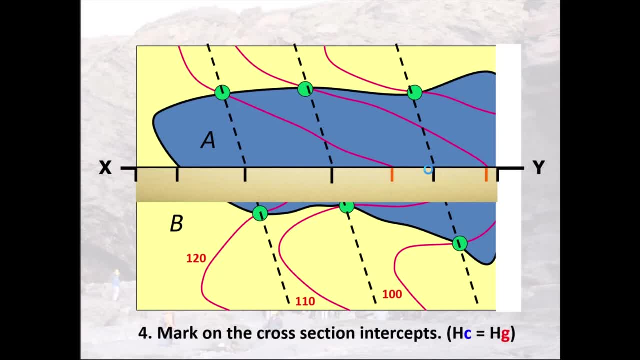 that's where our 100 structural contour. that's where our 100 structural contour intersects our cross-section. so then intersects our cross-section, so then intersects our cross-section. so then what I can do is use the red markings to. what I can do is use the red markings to. 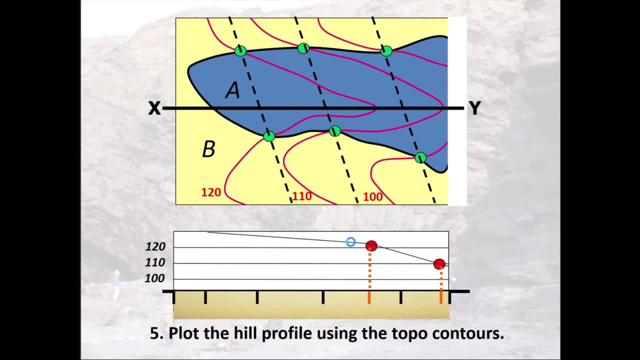 what I can do is use the red markings to draw a rudimentary Hill profile and draw a rudimentary Hill profile and draw a rudimentary Hill profile, and then what I can do is use the black. then what I can do is use the black. then what I can do is use the black markings where I've intersected the. 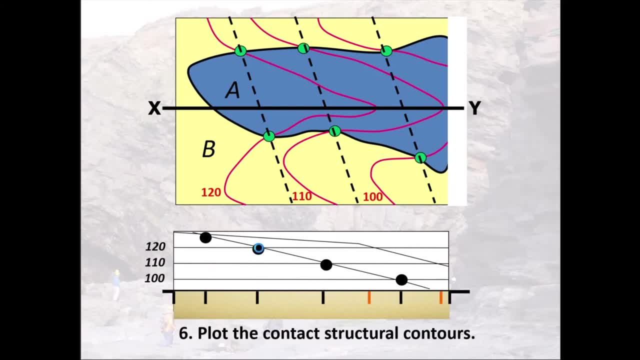 markings where I've intersected the markings, where I've intersected the contact at the ground surface, the contact at the ground surface, the contact at the ground surface, the contact at the 120 structural contour, 110. contact at the 120 structural contour, 110. contact at the 120 structural contour, 110 structural contour and 100 structural. 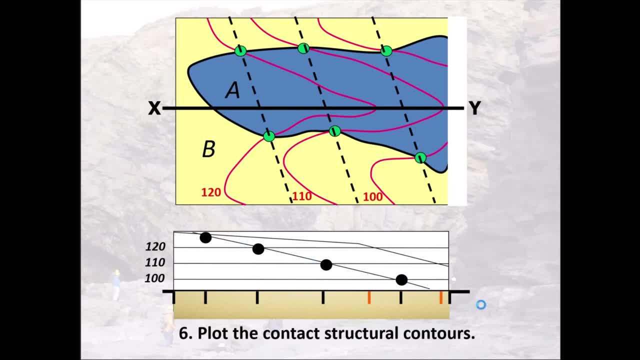